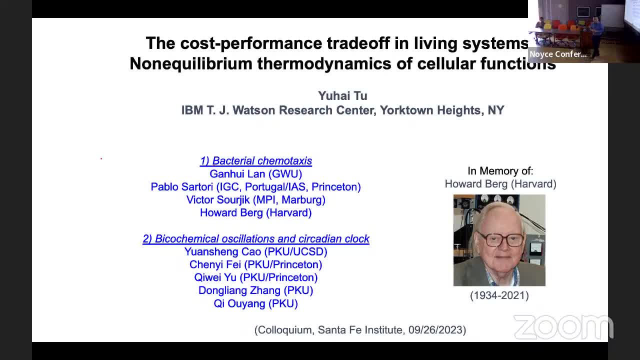 So I'm very happy to see this very nice environment finally. OK, so today I'm going to tell you about some work we have been pursuing for the, really for the last 15 years or so. So really try to understand the thermodynamics of small. 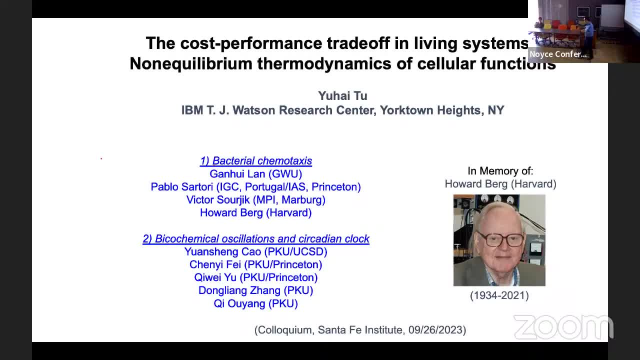 biochemical circuits, mostly in its thermodynamic property. We also worked on mechanism. That's a separate story we are going to tell you about. So the question we're trying to answer is: what is the cost and performance of these circuits Right? So we're going to talk about. 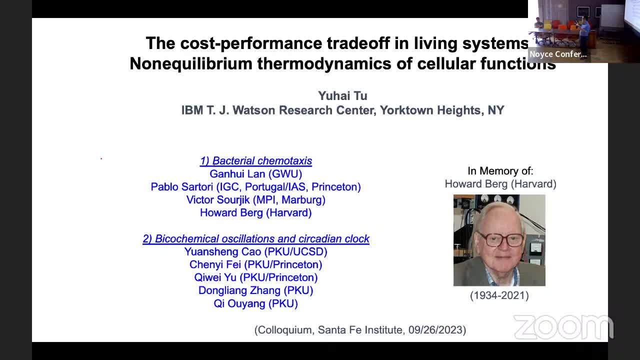 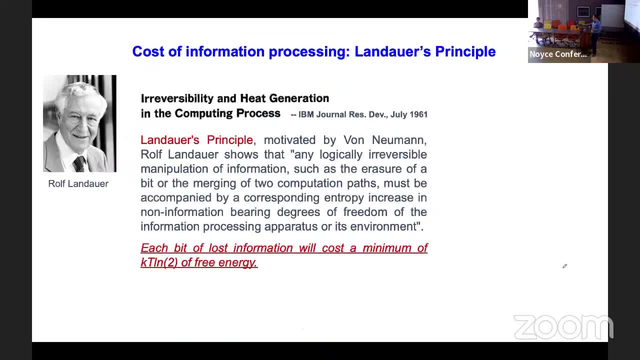 and performance of these circuits, All right. So the question we're trying to answer is: what is the cost and performance of these circuits? All right, So the question we're trying? Okay. so to that extent I talked about information processing. A lot of the processes I'm going to tell you about had a lot to do with information. 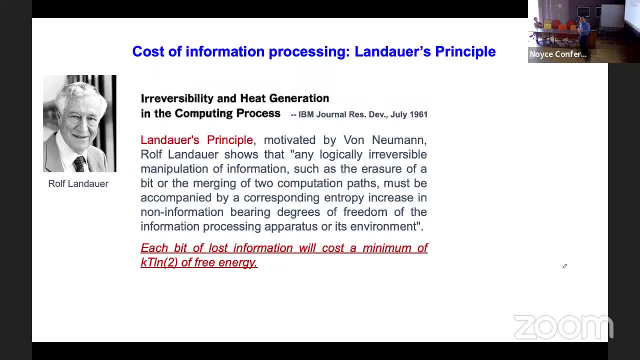 How did the cell deal with information? So this kind of question about how much does it cost to process information has been asked for computers, which is the machine that deals with information processing. For example, my late colleague Ralph Landauer has a principle named after him. 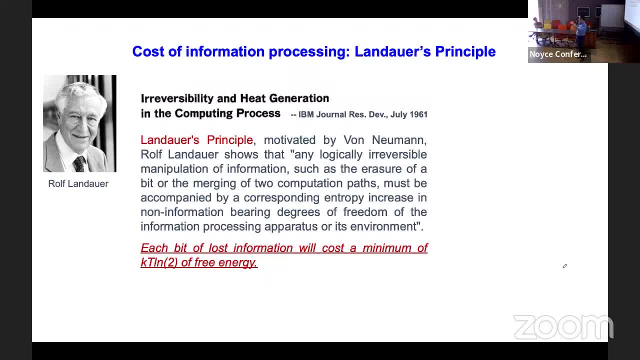 called Landauer's Principle. Now, how many people know about Landauer's Principle? Okay, pretty good. So Landauer's Principle is very simple. Ralph asked: how much information does it cost for a basic operation of erasing a bit? 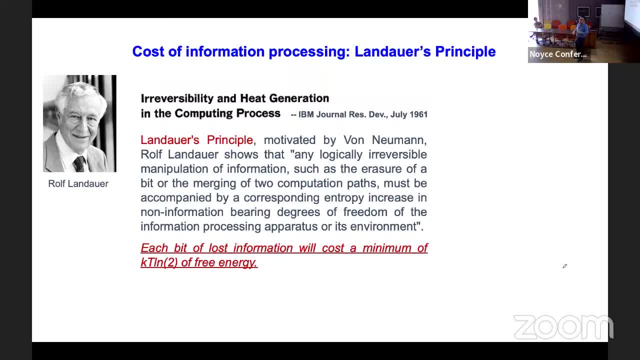 Write a bit and you erase it. That operation seems very innocent. but he says: well, to do that simple operation. it costs you at room temperature T. it costs you at room temperature T and the least minimum cost would be KT log 2.. 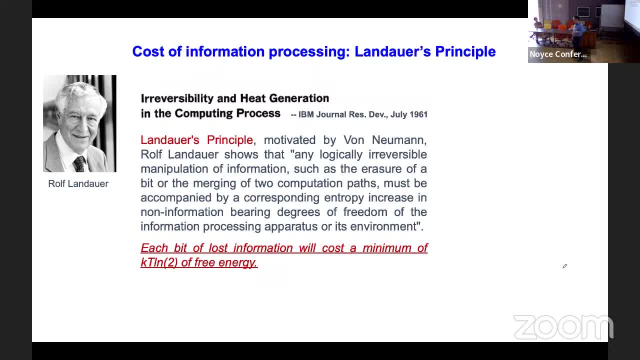 Log 2 comes about because your entropy, basically a reduction of entropy, going from two possible states to one state. That's basically the idea behind Landauer's Principle. It's a very simple idea. So I give you this because it's an example of people asking the question. 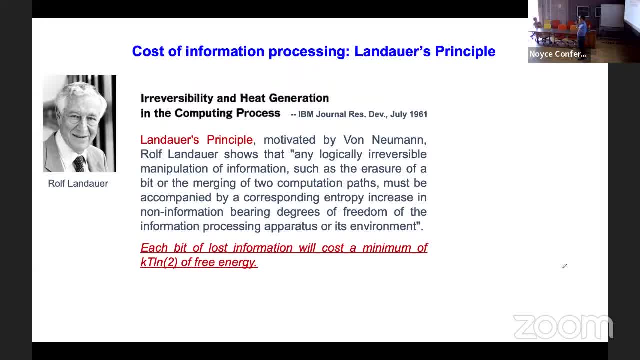 about energetics of particular operation that relate to information processing. So this, of course, basically erasure. yes, Does this depend on the size of the object that's holding the information? This is the lower limit, So this is an ideal situation. 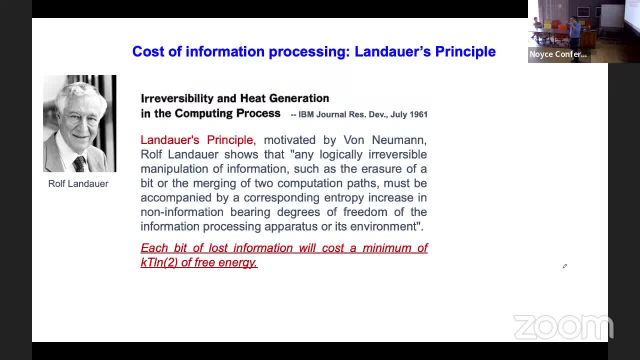 The structure he has, the landscape he has. it's basically double well. So you're basically going from double well to a single well and back to a double well. That's the operation. So the physical embodiment of that operation, of course, will cost you additional. 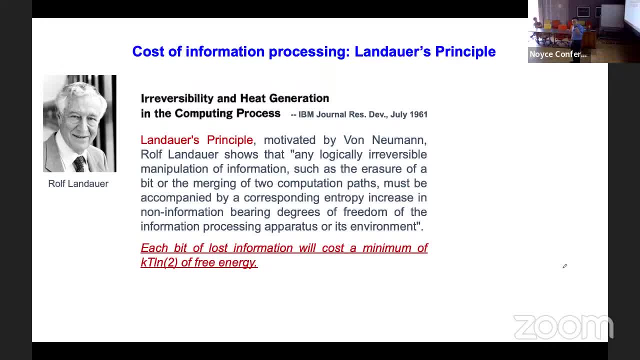 and it could cost you additional energy. But what he's saying is that the minimum is KT, log 2.. And if people have done experiments, actually achieved that limit in some artificial system itself, Yes, Similarly would it depend on what's the observer? 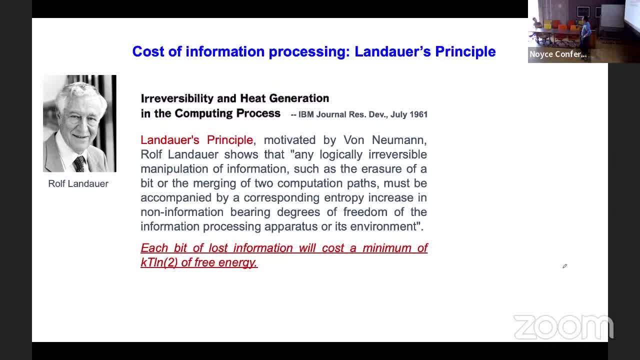 like, the observer needs to see the state right. So the observer also uses energy. Is that? I don't think it. yeah, that is not within the Landauer limit, But I think observer does cost energy, depending on the observation itself. 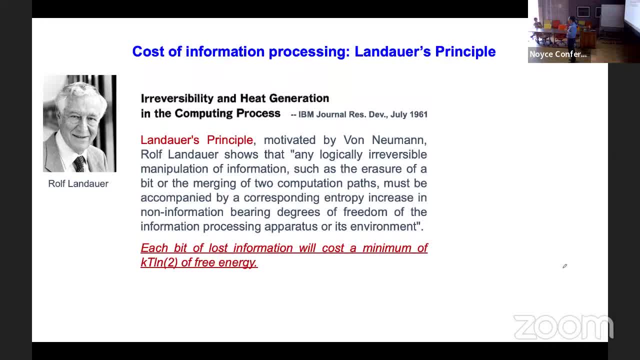 But I think another question that did not I did not tell you about is actually it depends on the speed. What it depends on is that how fast you want the erasure and the process happen. Actually, this is a very- it's a very- slow limit that actually you can achieve this. 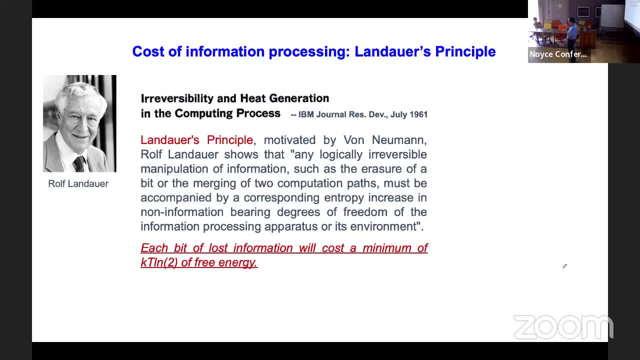 So if you want to happen in a finite time, then there's this. just corresponds to the infinite time limit, this KT log 2.. Yeah, Okay, All right, Let me move on. So this is just inspiration. I'm not going to talk to you about anything, about Landauer limit or anything. 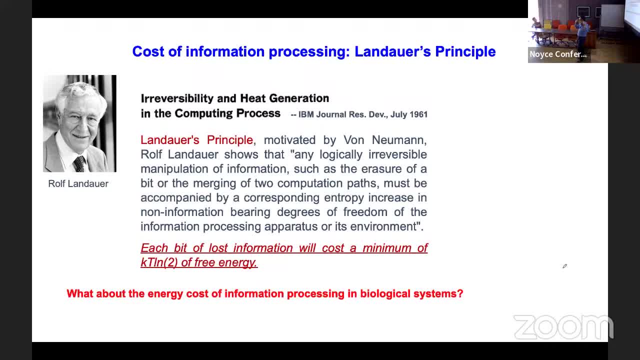 I'm just sort of inspire, inspiration from sort of the people thought about computation and the cost of computation. Now I'm going to take biological system as trying to do information processing and ask the same question: What about the energy cost of information processing? 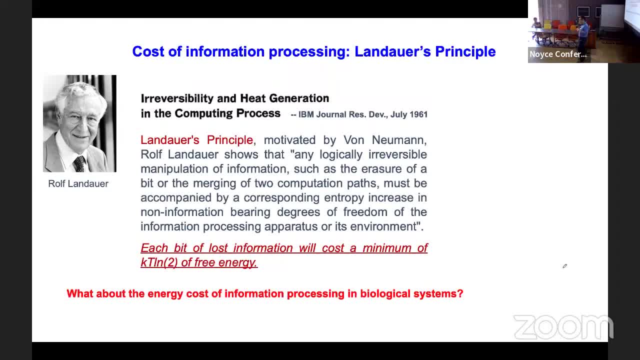 So here is a quote unquote: information processing. Probably the cell probably doesn't care about the bit or operation, but they care about their particular function, be it adaptation, be it synchronization. I can tell you about the other function that they carry out. 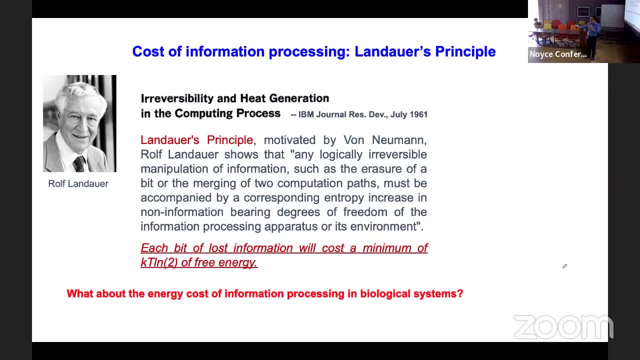 So, but you can still ask the question: how do you achieve these function and how much does it cost, Right? So we're going to ask the second question. So this is a question. again, it's very much central to computer scientists. 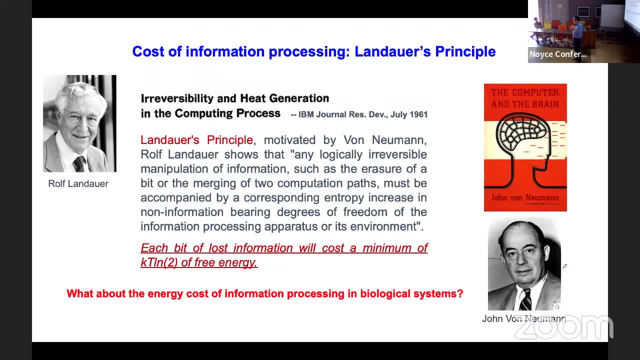 They actually really care about. you know von Neumann. just before his death he wrote the book Computer and the Brain. How many people read this book? Okay, so a little fewer people, Now that in that book he made a lot of observations comparing the human brain. 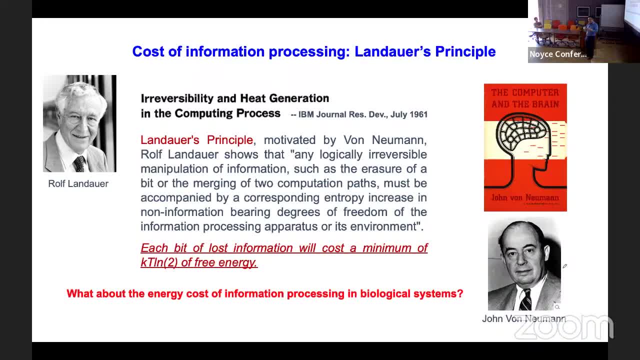 The fact that human brain, small the size and assumption, consumption of energy and so on. So what are the interesting observation he made, which I cannot seem to show, Anyway, the heat that one first makes? he made the observation that human brain cost 20 watts. 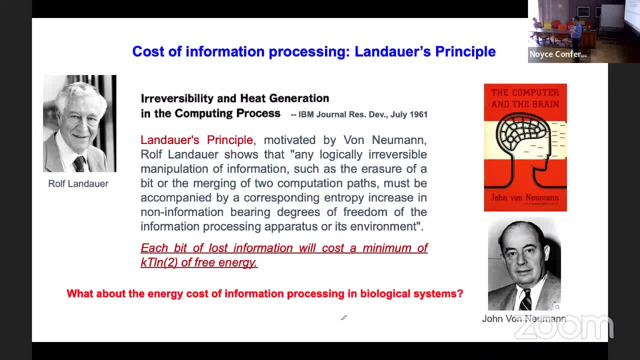 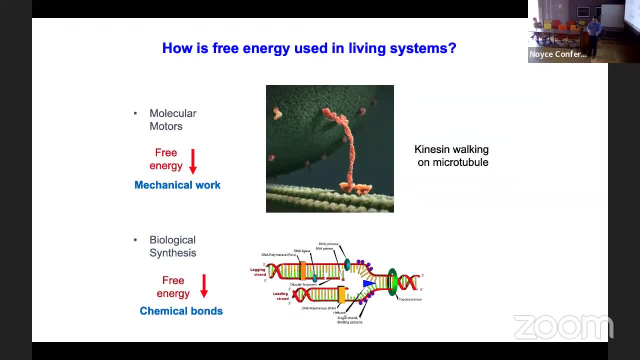 And yet even at that time, computer energy cost is tremendous, And nowadays it's you know so. so so this is pretty much on people's mind. So let's go back to living system. Let's think about how energy is being spent in living system. 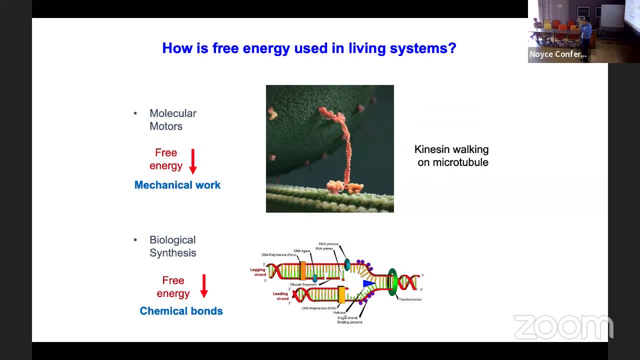 So this people, biologists, also care about this. The whole metabolism of living system is trying to harvest energy so that it can be used. Now talk about use is something that very important to biologists. So, for example, if you look at molecular motor, 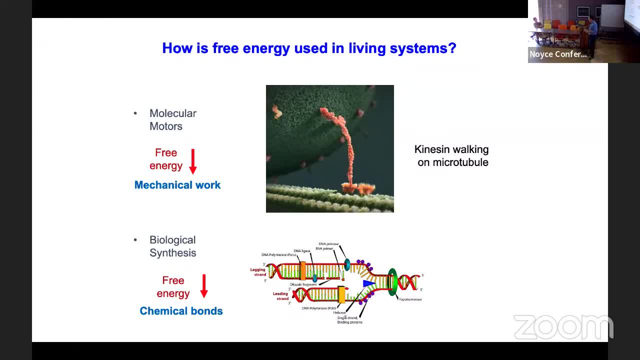 it uses ATP, burns ATP to carry loads. This is a a cartoon of Kinesin walking on microtubule, So it's actually burning ATP. It didn't show here, but actually ATP is constantly being built, being burned. 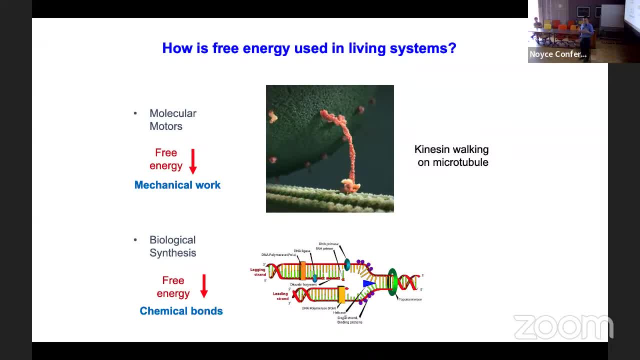 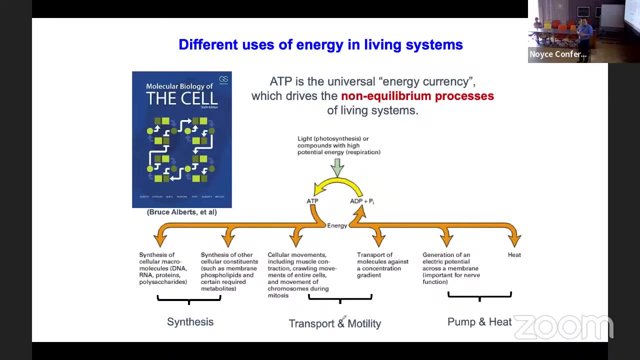 being hydrolyzed so that it can, you can do this. It also can be used for building chemical bonds, right? So you? so the all these building and synthesis and and mechanical motion costs energy. So, in fact, in this sort of Bible in molecular cellular biology, 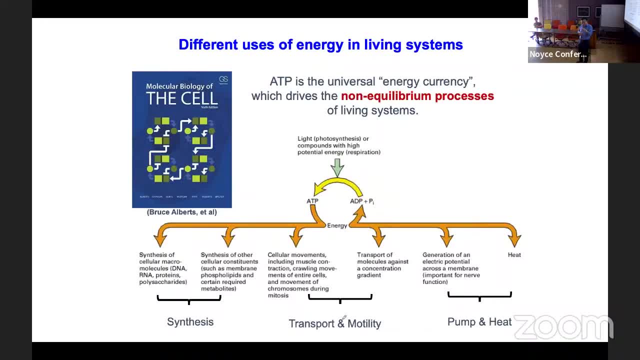 molecular biology, the cell by Bruce Albert. he actually listed all the way that energy has been used is used, For example, synthesis, right Transport, motility, basically plumbing of the whole system, growing things and and and doing plumbing takes energy. 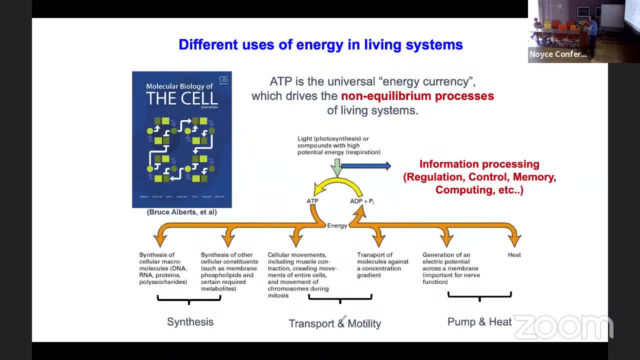 So what I'm going to tell you today, mostly it's about some hidden cost, which is actually very, very important. So what makes this living system very, very interesting is that actually all the regulation, all the control, all the like memory and computing in a single cell, from a single cell to a whole neural network. 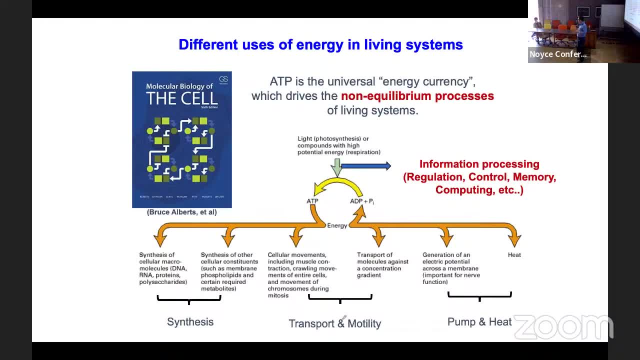 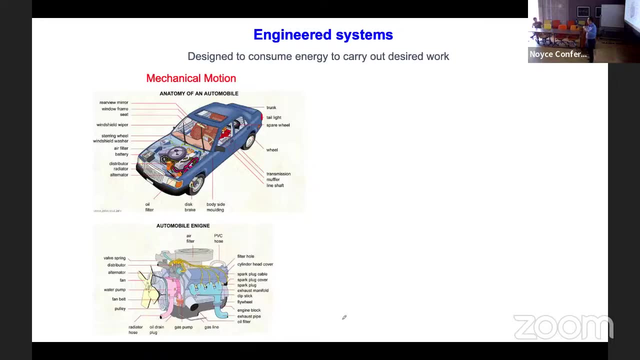 the brain actually costs energy And that's not necessarily part of these categories that Bruce Albert listed, And this is what we want to try to get to All right. So, thinking about systems, you have engineered system, you have the car, you have mechanical motion. 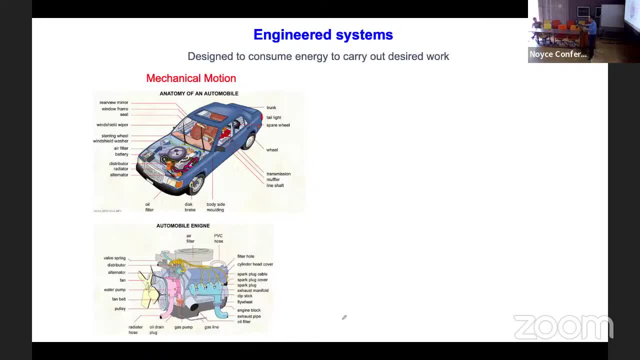 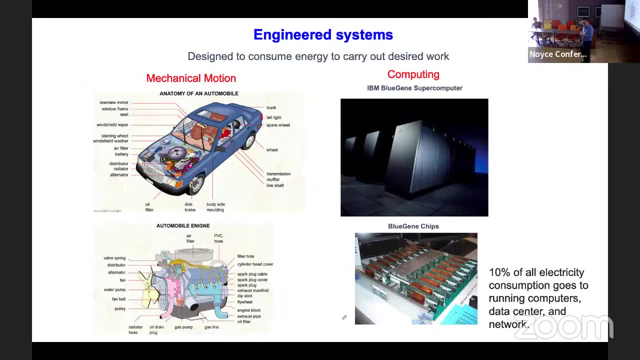 Of course you have to pull fuel, make it run, So you cost energy. but you also think you also know that computing also costs energy, right? So actually 10%- this is actually old statistics- of all electricity consumption goes to running computers. 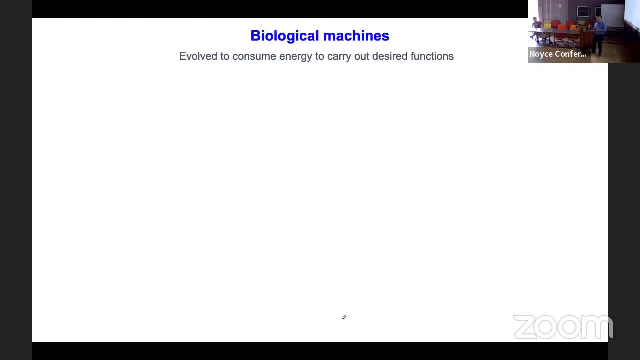 So they're just very stunning statistics. It's growing right. Of course, biological machine does the same thing. So if you think about the motor, I told you before that here's, here's a Fagella motor. It burns on. 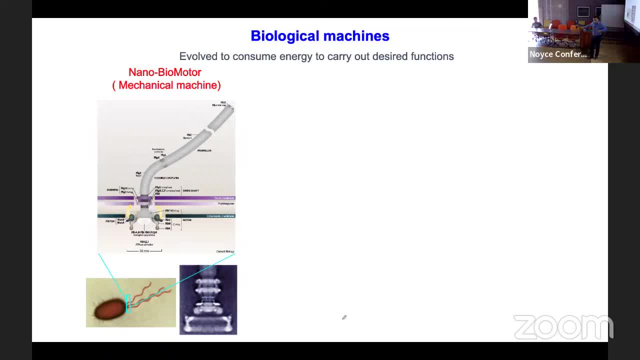 not on ATP, but it actually burns, a potent motive force which is maintained by ATP hydrolysis, But anyway so it. a biological machine also costs energy, but the unit, the currency of energy in biological world is ATP or other high energy molecules and other. 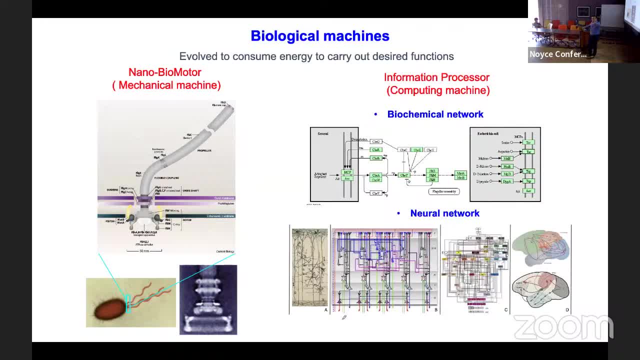 So the right hand side category, sort of you, you, you, you. you probably heard about biochemical networks. These networks are protein interaction with each other. This network and circ, we'll call it molecular circuit and also neural circuit, like this: 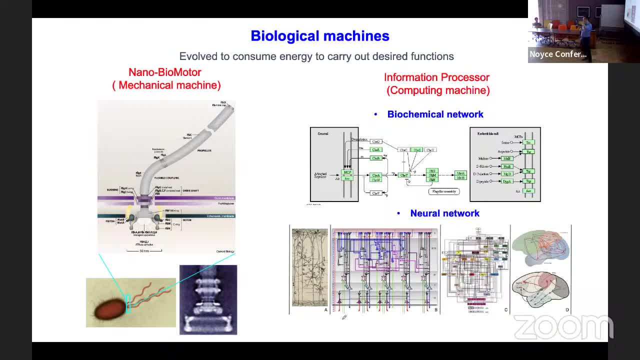 It all costs energy to run these circuit And the purpose of these circuits are or either regulation, controlling it, not necessarily moving things around, that, that, that, that the kind of thing that you are directly associated with cost of energy. So these are all on the right hand side. 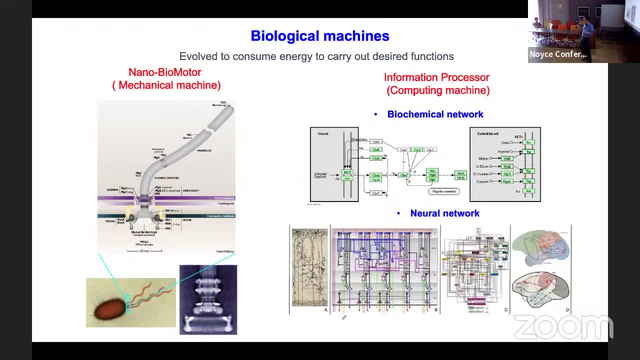 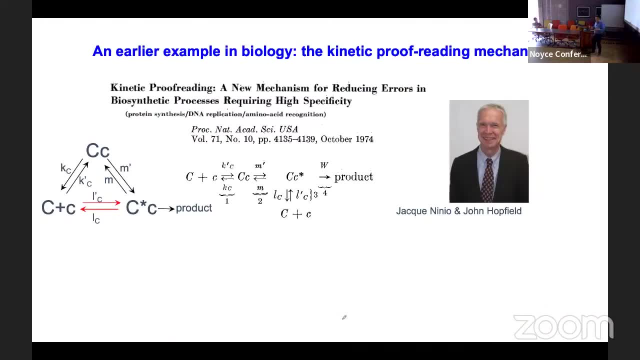 I will characterize as the computing or or information processing, And this is the part we're going to try to understand how that, how much energy did it cost for these circuits? So so what? what? give me an example, You can ask me what. 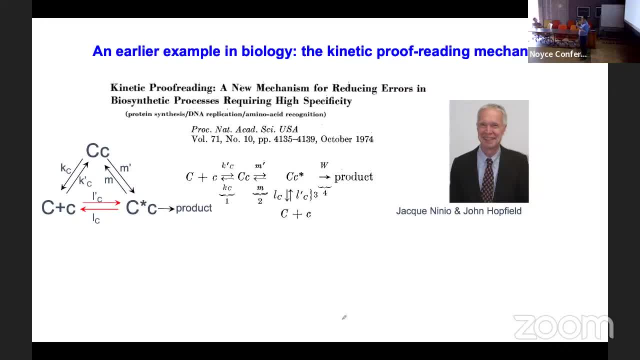 what? what is it all about? Can you give me a specific example of how, what, what, what, what I'm talking about? Well, kinetic proofreading. So this is a scheme that proposed by John Hoffield and Jack Nino some 40 years ago. 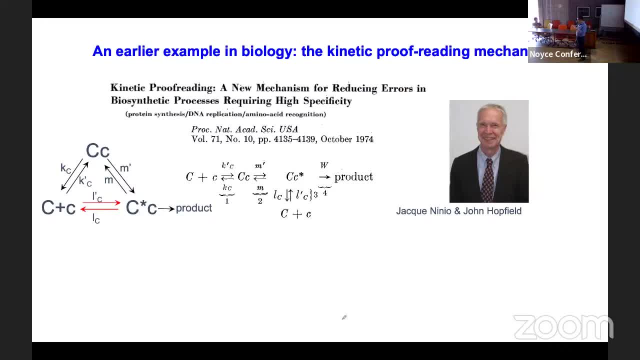 roughly that. try to understand the, the error rate, The error rate in DNA replication or other biomolecule synthesis. So if you just look at the base pairing energy of the correct base pairing and incorrect base pairing there is an energy difference That correct base pairing is. 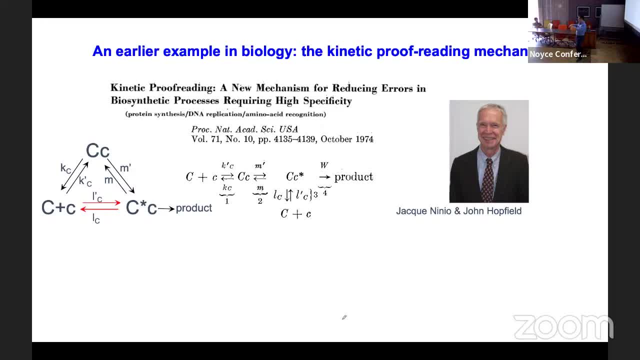 has all lower energy. But if you just raise to the, you know, using the Boltzmann factor, you find that energy difference between the correct base pairing and incorrect base pairing only give you 10 to the minus 3 error rate, Whereas in the real life. 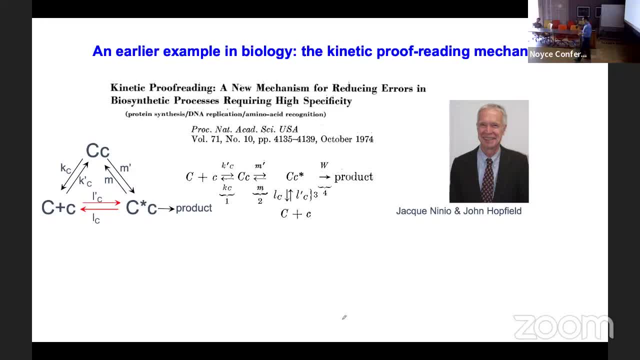 you get much less than that: 10 to the minus 6 or and and less. So what's going on? So obviously biology has to invent some way of correcting error, right? So, and Jack John John Hoffield actually proposed one very simple way. 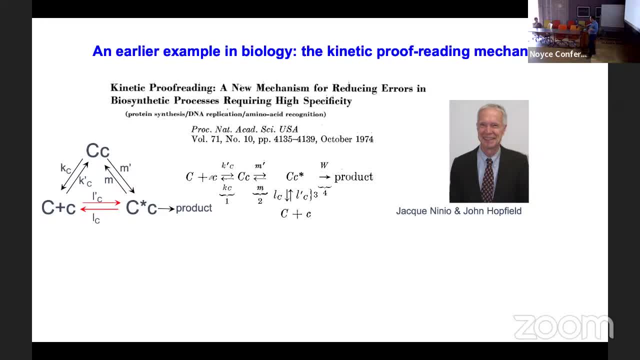 So here is basically a very straightforward: If you add another little base pair, it actually pair with it and then becomes product and you can move on right. So what he did exactly: just adding another feedback loop or or backflow, Basically from the group. 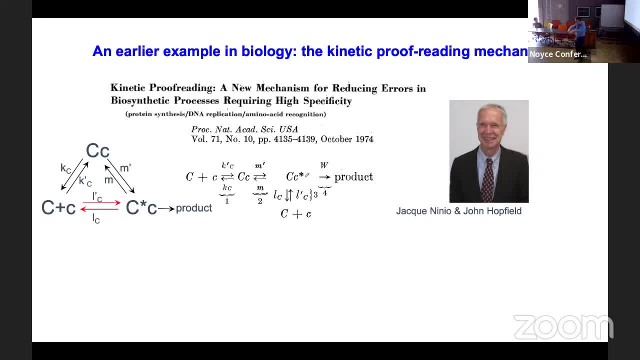 from the already synthesized pair. you actually shake it and you shake it with some, with some ATP consumption, So that actually there's a there's a finite chance for you to break away so you can restart the process again, If you restart the process again, 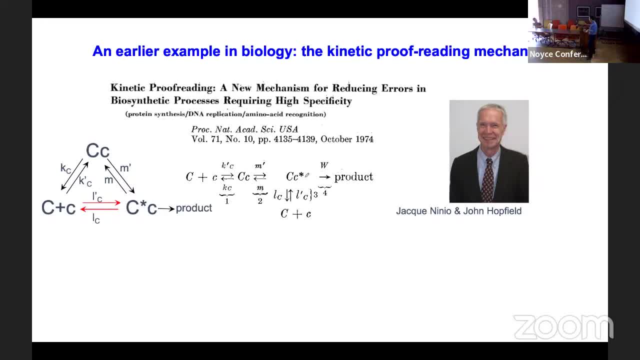 and then the error rate will be going from original error rate of P to P square If you do it twice right? That's just, and and that's the. that's the kinetic proofreading mechanism that he proposed, Right? So how many people had heard about kinetic proofreading? 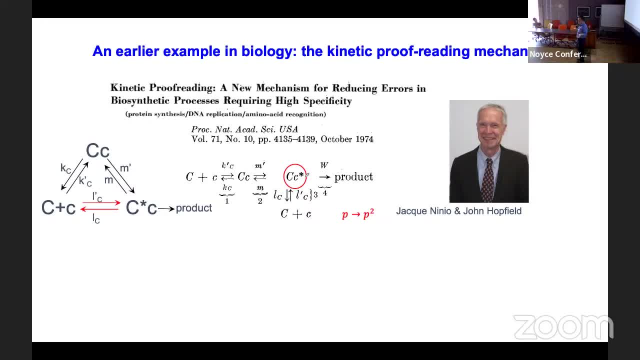 Okay, So so that's actually very nice mechanism. So this is belong to the mechanism part, So I'm talking about how much. then actually comes out Another very interesting paper- not too many people read about it, but by my, one of my colleagues still living. 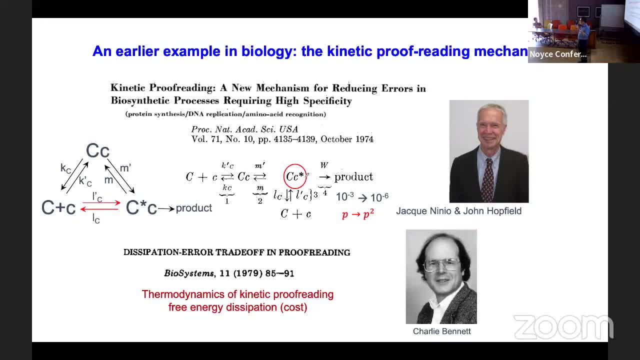 Charlie Bennett. Everybody knows about Charlie from his quantum computing, quantum teleportation- How many people know about? he did work on kinetic proofreading. No right, Oh, you did. Okay, You do Now. he right after. 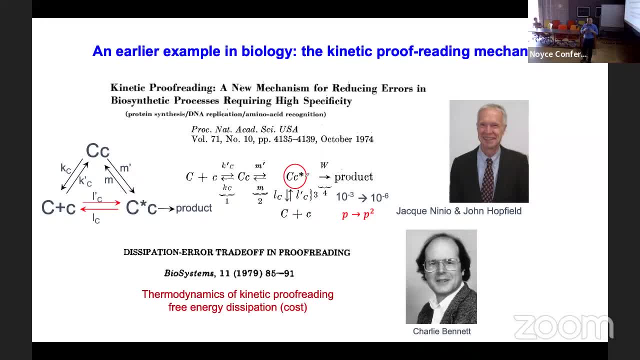 a few years after the kinetic proofreading was proposed, Charlie wrote a paper in biosystems about dissipation: error, trade off improving. What he showed in this paper is that actually, indeed, it costs energy to do it, to do the error, the kinetic proofreading- and the amount of energy cost depends on the speed of replication. 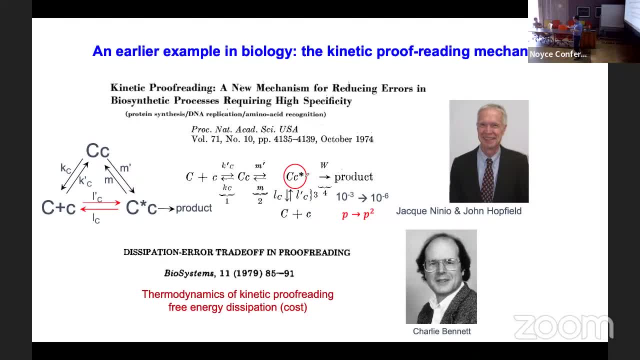 and the error, the desired error rate that you at the end, Right. So it's very nice paper I'd suggest. I mean I really would recommend, if you're interested to read about this paper. Okay, Now in the title, 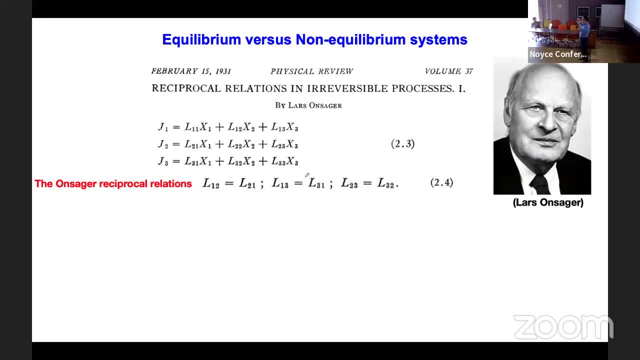 I talked about equilibrium, non-equilibrium, physics, non-equilibrium. you know thermodynamics. What do I mean by non-equilibrium? How do I know the system is out of equilibrium in a biochemical reaction system? How do I even know that it's out of equilibrium? 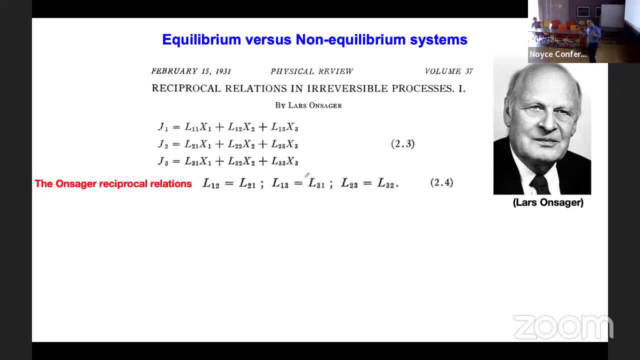 Right, So actually you don't have to look very far for a definition. Lars Anzager for the prize. I won the name after him actually in his Nobel Prize winning paper. this is a paper about reciprocal relation which won him the Nobel Prize in chemistry. 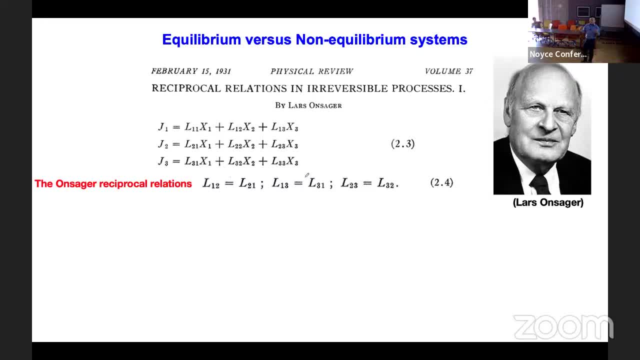 not in physics, in chemistry. He actually was looking at reciprocal relationship in system just a little bit away from equilibrium, Right. So he can do linear perturbation theory and all that stuff. What he found is that in the equilibrium system, if you perturb it. 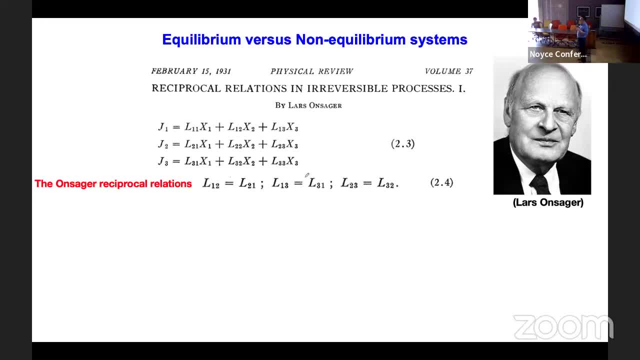 and and the perturbation can be. the response of the perturbation can be described by these coefficients. The Anzager reciprocal coefficient L12 is the: if you perturb in the two variable, two X2, what is the response in variable X1?? 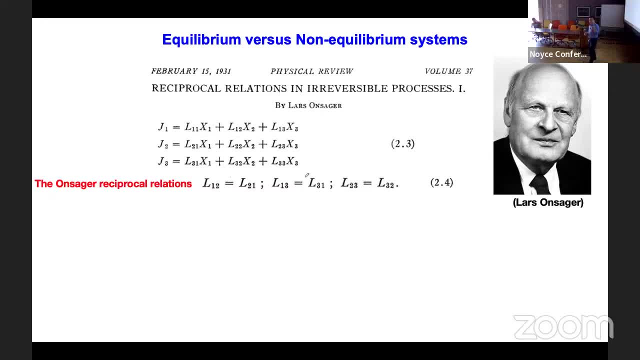 Right, So the cross relation. So what he found is that in the equilibrium system it has to be symmetric. L21 is equal to L12, and so on. So you have, you can imagine, this response: matrix has to be symmetric matrix. 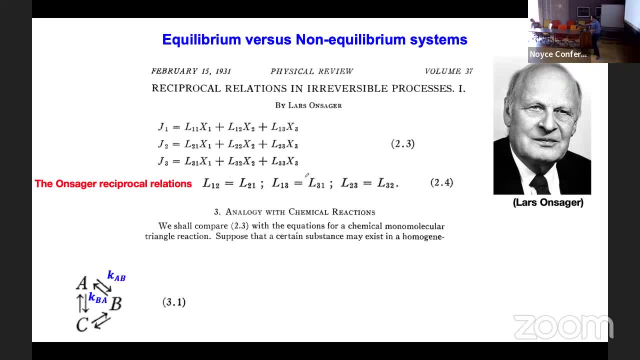 Now he so again. not too many people probably read on to his paper In in section three of his paper he made an analogy with chemical reactions, which is what we want to be studying. So in chemical reaction the analogy he made is basically: 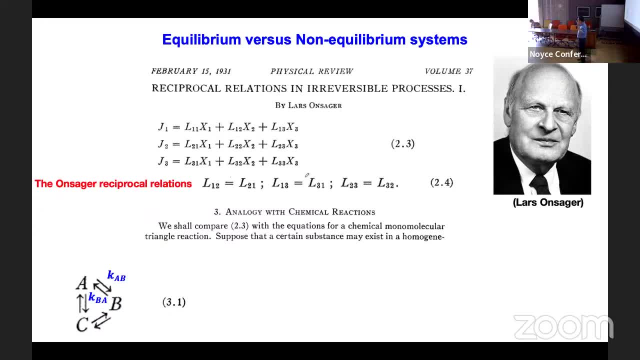 okay, you have three species of chemical state- A, B and C- And they are transitioned between any pair of them. So, for example, from A to B you have KAB, from A to B, you have KBA. 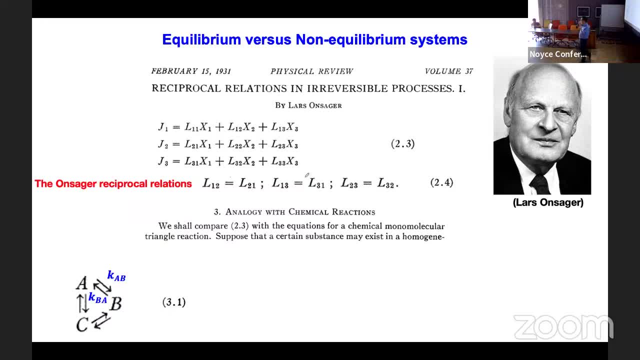 K are the reaction rate Right Now. equilibrium system satisfy detail. balance, Another very important concept In the equilibrium system. what does it mean? It means that the net flux, probability flux of going from one state A to B. 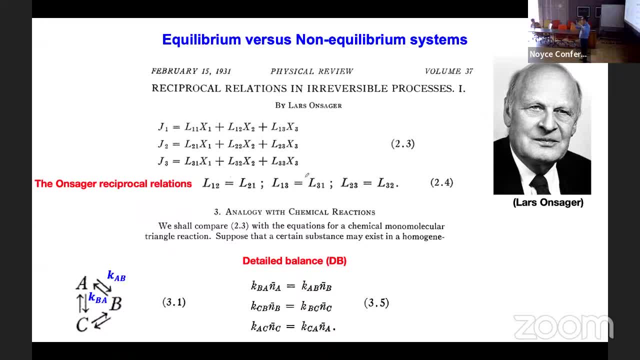 has to be the same In steady state, has to be the same as the flux going to B to A. So the KAB times, the probability of in A and A total, is equal to KBA AB times. NB Right. 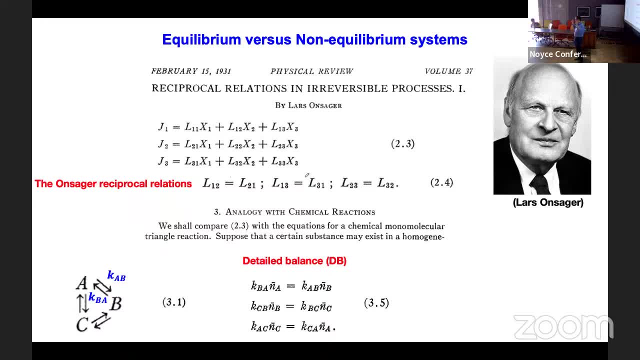 So so on. So that's the detail balance. Now, from the detail balance, you multiply the three equation together. N drops out. What you obtain is a relation between all the Ks. So this is what I call the cycle rule. 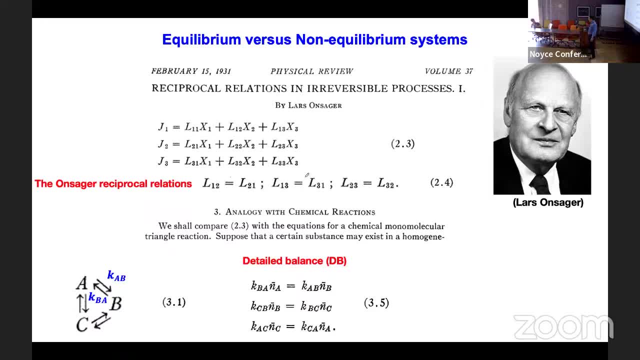 Meaning that if you multiply all the rates going, let's say clockwise KAC times, KCB times, KBA, it has to be the same. So if you multiply all the rates going, let's say clockwise KAC times, KCB times, KBA. 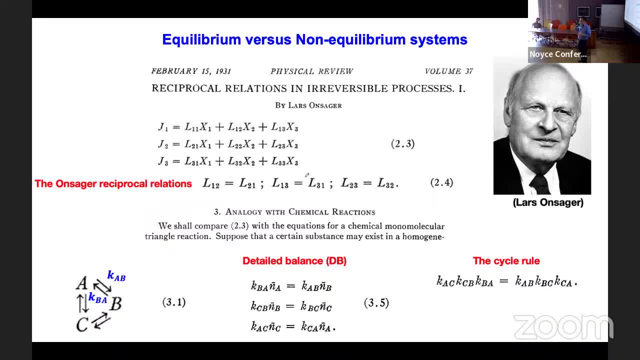 it has to be the same. So if you multiply all the rates going, let's say clockwise K, it has to be equal. I only, I only copy. this red part is my writing. I only copy and paste what he wrote. 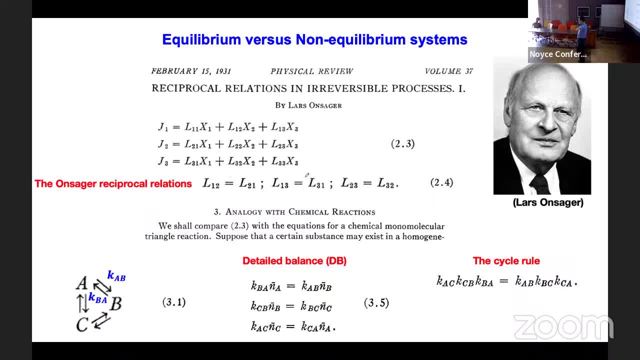 in this paper, Right? So that's the cycle rule. So in the Euclidian system, the all the Ks. if you multiply all the K, all the reaction rate in one direction has to be the in any cycle. 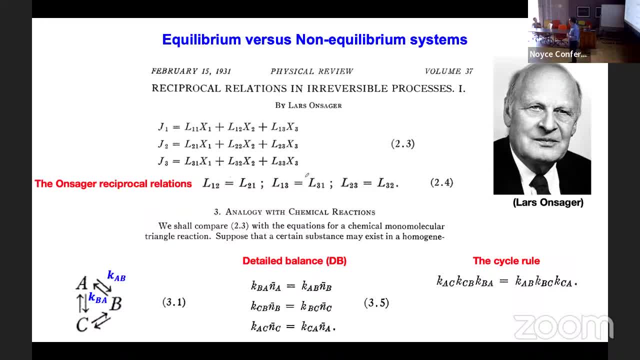 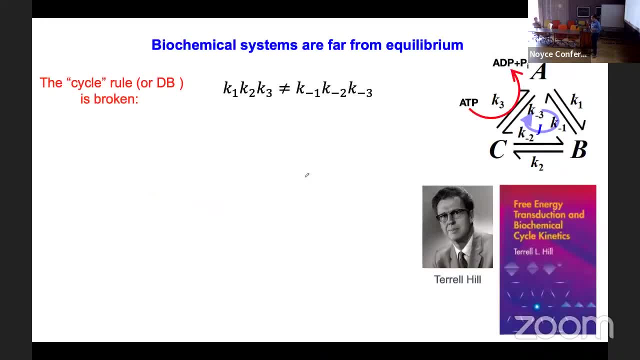 has to be equal to the product of reaction rate from the other cycle For every cycle. Okay, So that's the. that's the Euclidian system. Now, non-Euclidian system is is exactly that. It's exactly breaking. 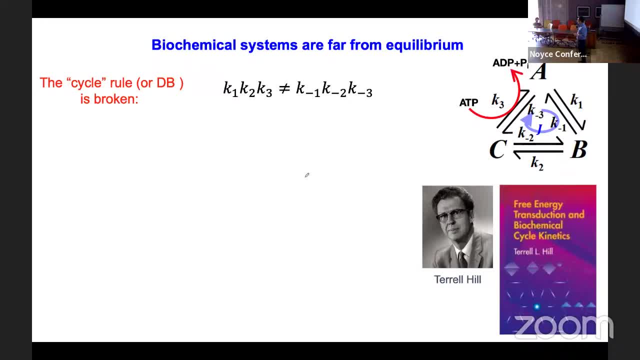 if you break the equality in any of the cycle in your system, then your system is out of equilibrium. Out of equilibrium doesn't mean you don't reach a steady state. you do reach a steady state, but that steady state is called non-Euclidian steady state. 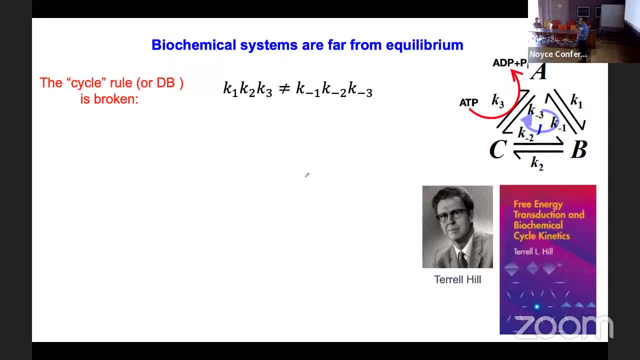 which will have interesting properties. that, as we later on show, has a lot to do with the function. you try to, so you can break it. So how do you break it? You break it by enhancing the rate, in this case. 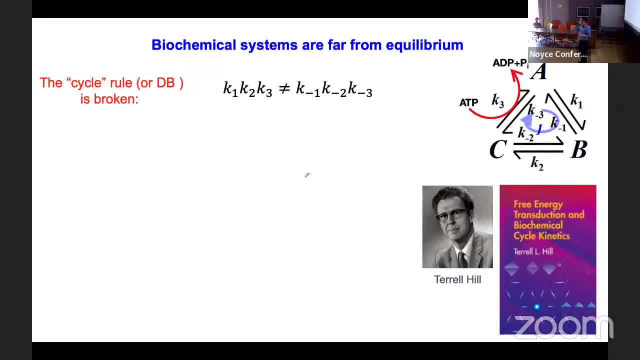 in the right hand side, from A to C or C to A by coupled reaction, where you say ATP hydrolysis, Right, So ATP hydrolysis of course releases energy, so that particular reaction rate. 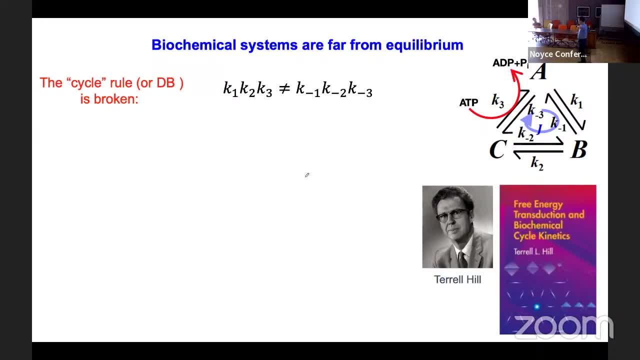 is enhanced And, as a result, you have this inequality Right. So you can couple your ATP hydrolysis to any of this in this reaction so that the break detail balance Right. That's just the way to. 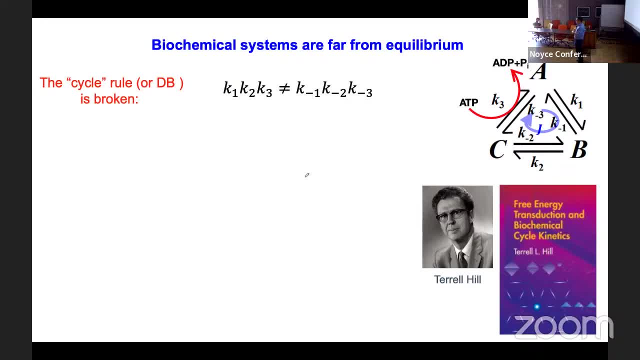 go from equilibrium system to non-Euclidian system, But exactly how you break it and where do you put the energy, how do you use it to achieve the function you try to achieve, is what we're gonna talk about. 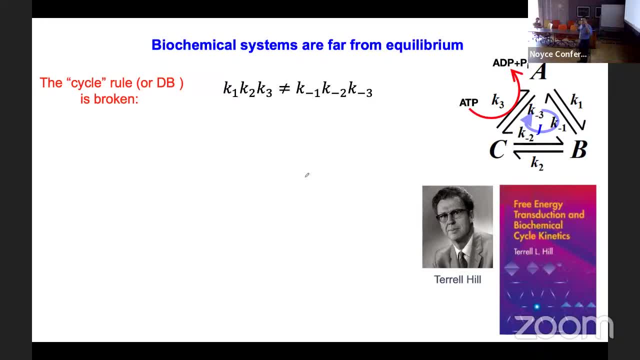 So in this business about free energy dissipation, transduction and biochemical psychodynamics, again I mentioned this book by Terry Ho. Again I'm asking how many people know about Terry Ho's work in this. 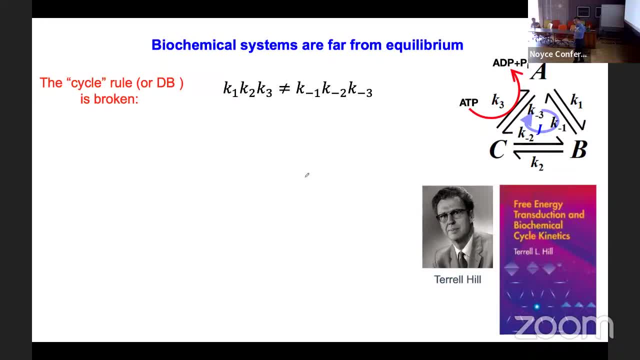 in this domain. Two or three, Okay, so that's giving less and less. So this is really the unsung hero. He is really the unsung hero for the whole non-Euclidian thermodynamics business. He's really the first one to realize. 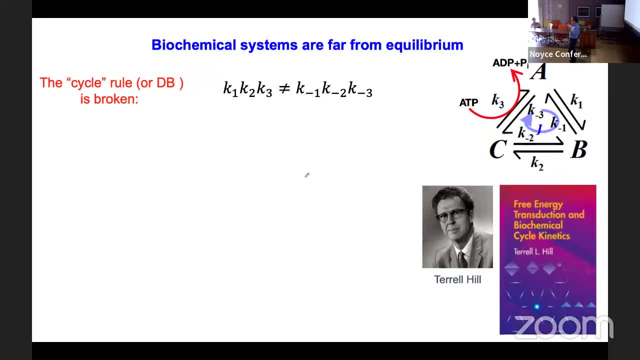 hey, we can connect the dissipation with actually the function. But of course at his time the only system he studies are motors. So that's what his limitation was. But anyway, the whole formalism was laid down. 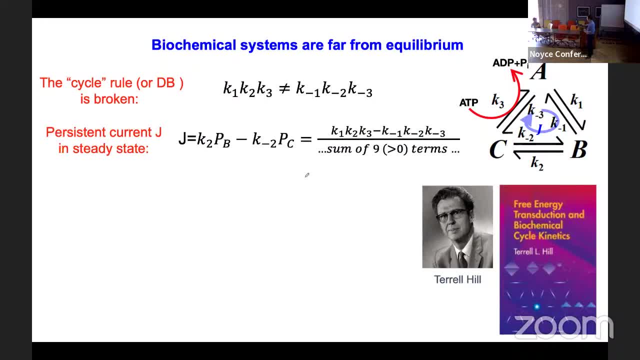 very beautifully in this very nice little book. For example, one of the characteristics of this non-Euclidian system is that remember I said the cycle right By breaking the cycle, rule the equality if you have an inequality. 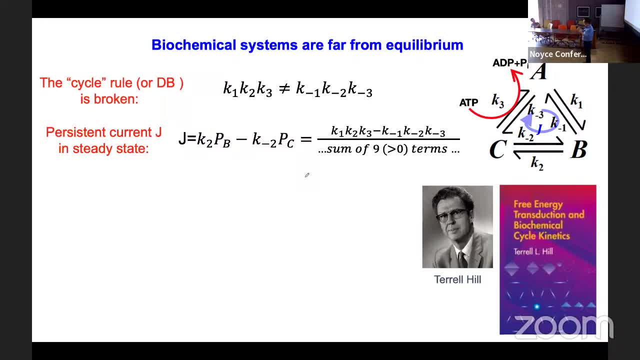 what happened is that in the steady state right, Not the transient state- in the actual final steady state you have persistent current going through the cycle, Whereas in the Euclidian state, where each cycle rule is satisfied, the current is zero. 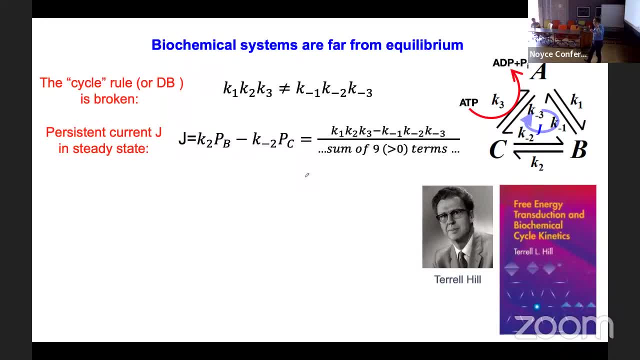 Not only can do that, in the simple system you actually can compute the persistent current probability, current in the steady state, the J, And you can compute it. it's basically. you see, the right hand side, the numerator. 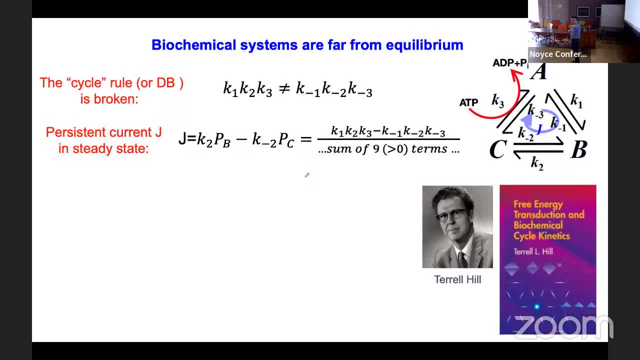 is basically K1, times K2, times K3, minus the reverse. So in the case where they're equal, of course the J equals zero, right. So it's a very nice demonstration of how. breakdown of detailed balance. 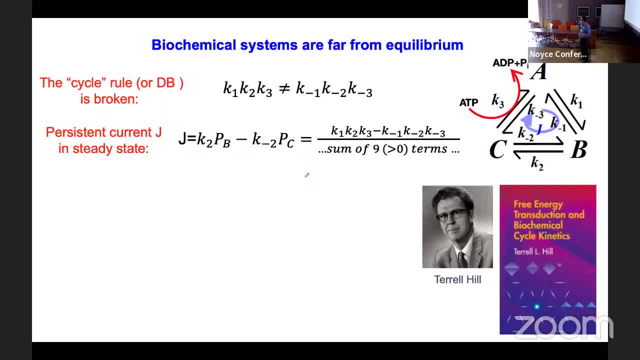 lead to breakdown of cycle rule. breakdown of cycle rule leads to persistent current probability, current in the final steady state of the system, And from there you can also compute a thermodynamic driving force, delta mu, which is basically. 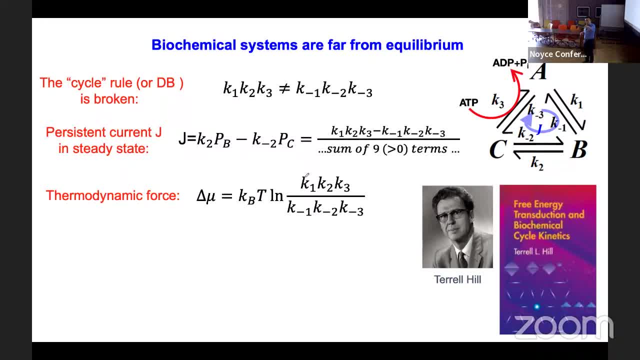 the logarithm of the product, the counterclockwise, divided by the product the clock counterclockwise and the multiplying delta, mu times J give you the dissipation rate. This is how much energy is dissipated. 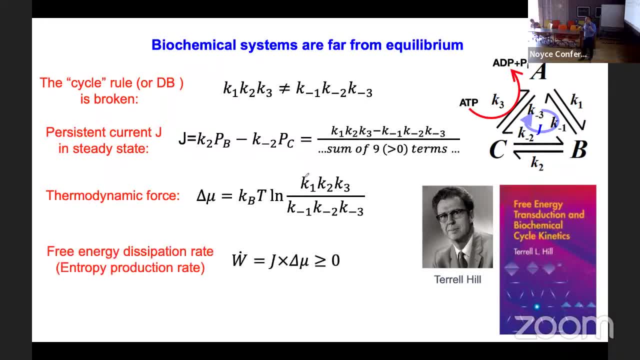 Or in other business people call it entropy, production rate Right. So if you're going to dissipation rate, you're going to have to, you're going to have to, you're going to have to, you know dissipation rate. 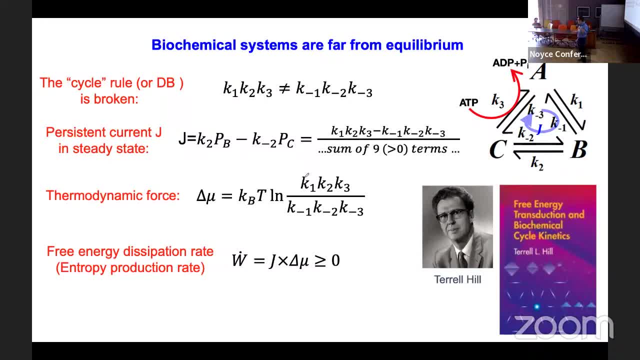 is basically J times delta, mu And it's easy to show delta, W, dot. the rate of dissipation is positive, definite Right. It only becomes zero when J goes to zero, When, in the equilibrium case, 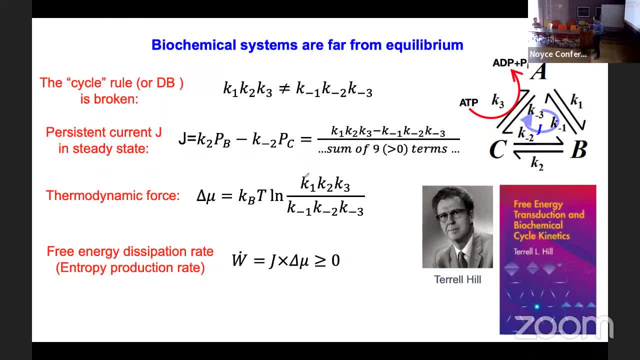 Cannot be negative. All right. So this is a sort of general background. So, in other words, continue continuous energy dissipation or power consumption is needed to maintain a non-equilibrium steady state. The steady state comes. 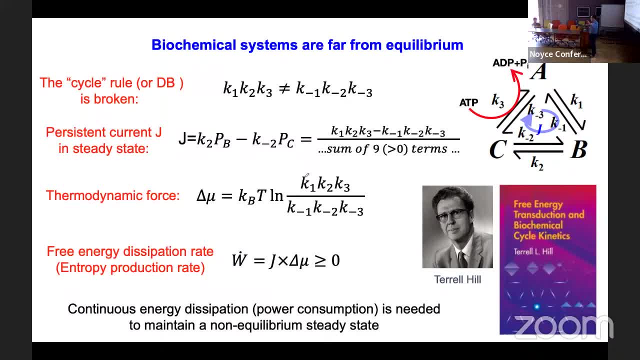 with a price, And it is that steady state that we actually can relate to. the non-equilibrium steady state can relate to particular function And that's how we're going to build the function relationship between the cost and the function. 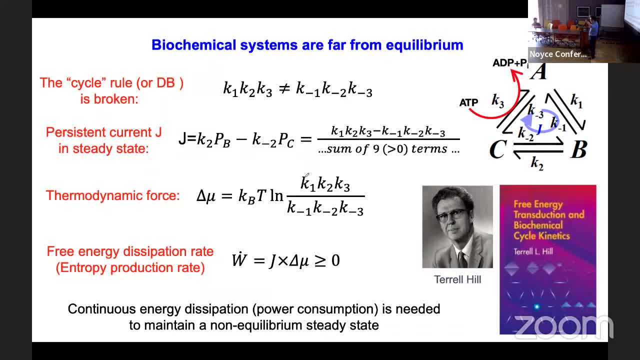 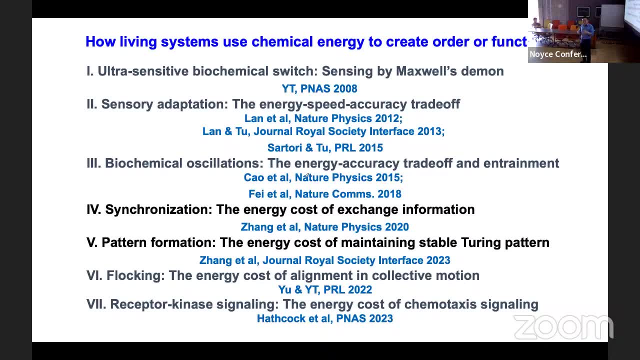 All right. So along those lines, you know, as I said, in the last 15 years or so, this is a long journey and still going. We have done a number. look at a number of systems, including. 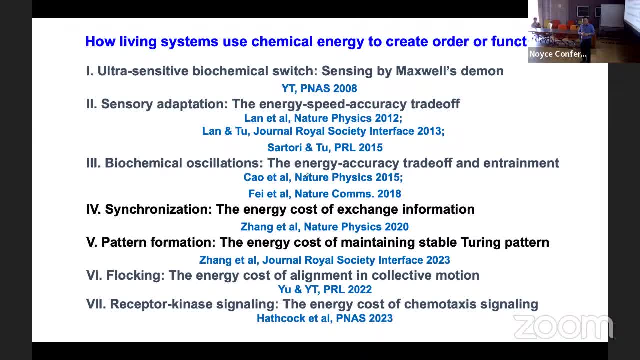 ultra-sensitive streams And you know we have. we have ultra-sensitive switch in bacterial flagella motor to sensory adaptation, to biochemical oscillation synchronization pattern formation. These are the two I'm going to tell you about. 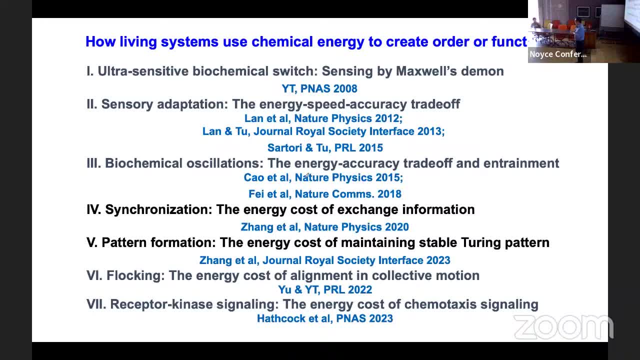 and also about flocking. So you mentioned the work that we did many years ago about flocking. Actually, it turns out that's a very typical non-equilibrium system. You, you will not have long-range order. 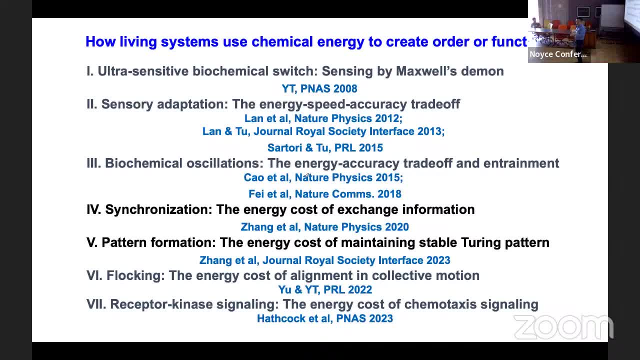 in low, in two dimension, without dissipation, And we will be able to relate the dissipation, which actually the order. actually pretty nice, satisfying work after all all these years. And also we work, we continue working on. 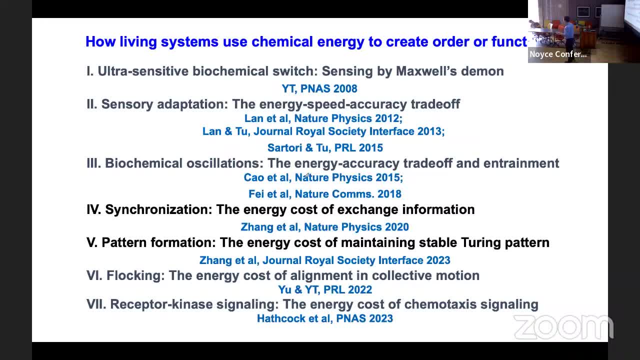 bacterial chemotaxis. So this last piece of work was I talked about earlier this year. It's coming out in PNAS, maybe tomorrow. Okay, so so, but today I'm going to tell you two systems. 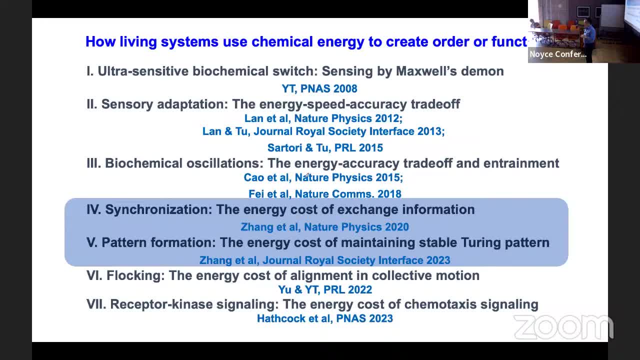 that I took I I I promised in my abstract. One is about synchronization of molecular clocks, So this has to do with temporal order. So I I picked this two because of the order in. 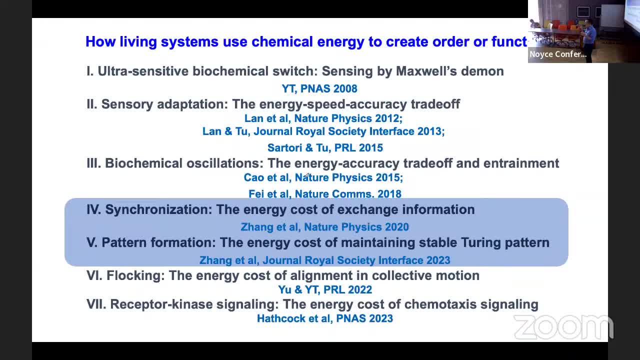 so what order? Order in space and order in time. The first one is about order in time. How do we have an arrow of time in non-equivalent system, in living system, molecular system? The second one about pattern formation. 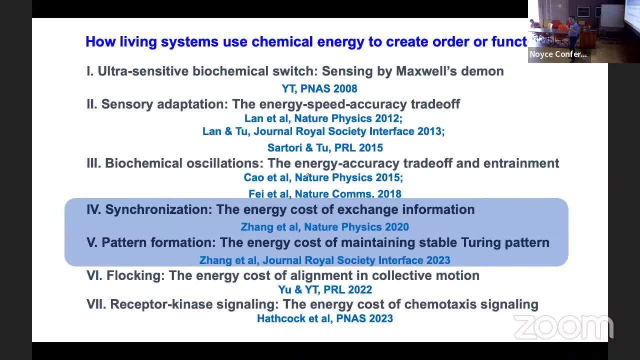 is about order in space. How do you create order in space? And in this case, we are we. we worked on, basically, energy cost of Turing pattern. Okay, All right, Let's dive in, Okay. 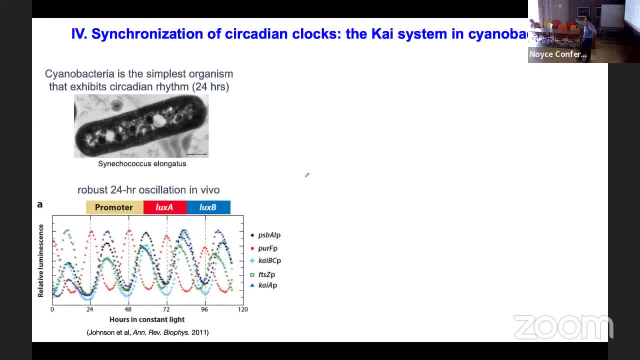 So about synchronization of circadian clock? This is a large subject. I'm not gonna go into all the details about the molecular details of how this clock works, But suffice to say this is probably the most beautiful. 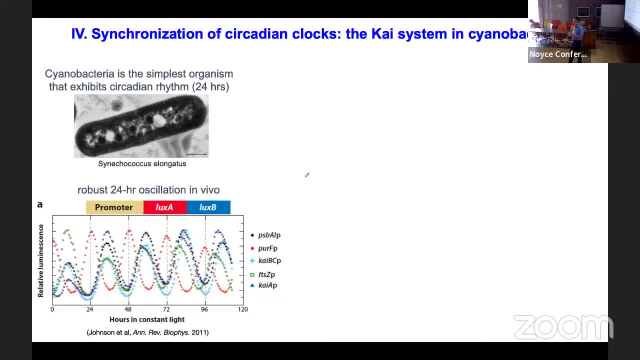 circadian clock- Simplest. This is the IZ model, if you want, of of circadian clocks- Has three components, So let me just show you It's it actually have circania cyanobacteria. 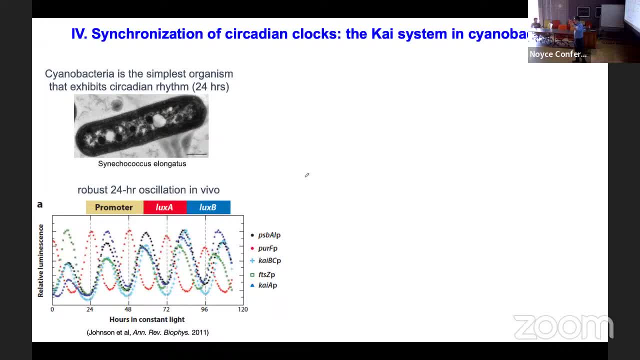 organism Or other circadian clock happen in like human and animal. It happens in high. animal has to do with interaction between neurons and inside the cell. Also had to do with a complicated you know. 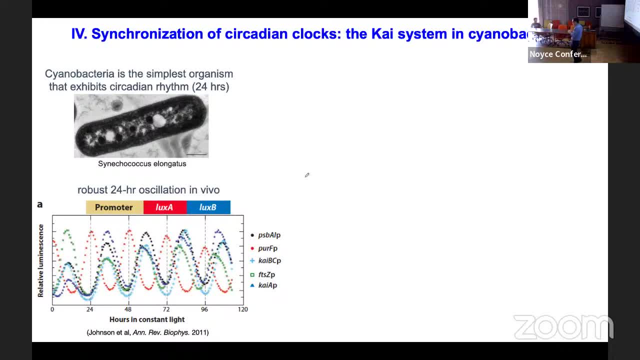 different gene, interaction between different gene, and and and protein product and so on. Here it's really down down to the core. This clock, 24 hour clock- is really a purely protein. it consists of three protein. 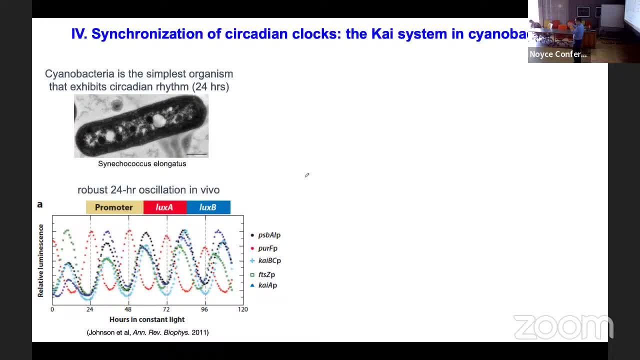 And the main part is really the chi C, the hexamer of the. it forms a hexamer. That's the. that's the clock And it. it just lower left. it just shows you the clock actually. 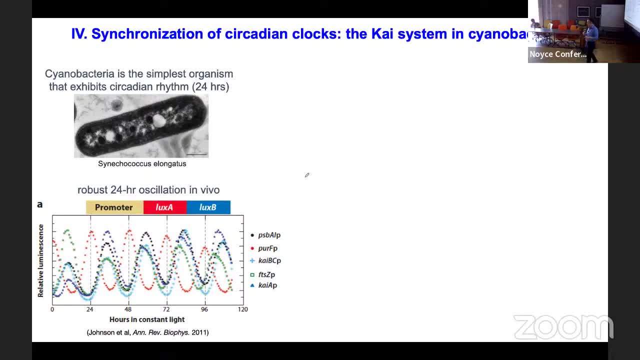 controls all gene expression for other protein right Robust 24 hours in vivo. Now the the field really took off in 20 years ago- roughly 20 years ago, because of condo, was was able to. 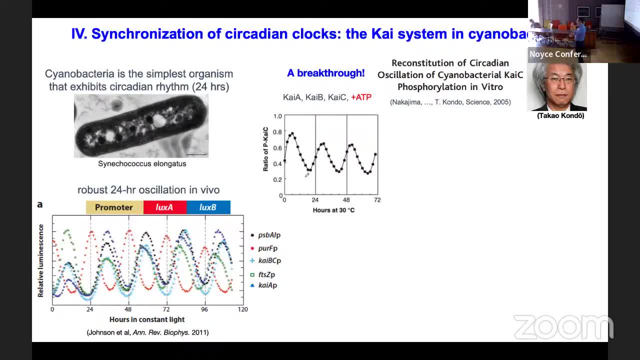 reconstitute the whole clock in a test tube, right? Like I said, there's three type of molecule in protein: chi A, chi B and chi C. who was able to synthesize it now put in the test tube. 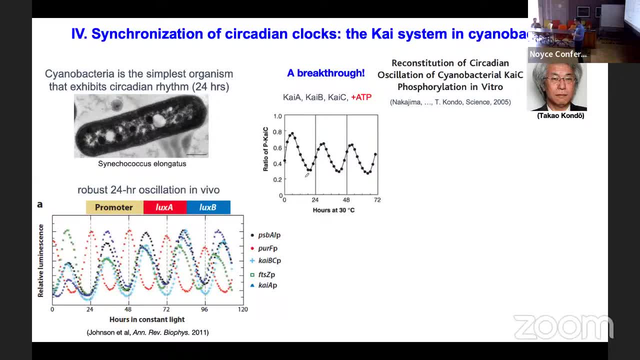 It oscillates. No, You have to add ATP, of course, add energy. So you clock any clock. even this clock runs on a battery, right? So you have to add energy. So this is the part I'm gonna tell you about. 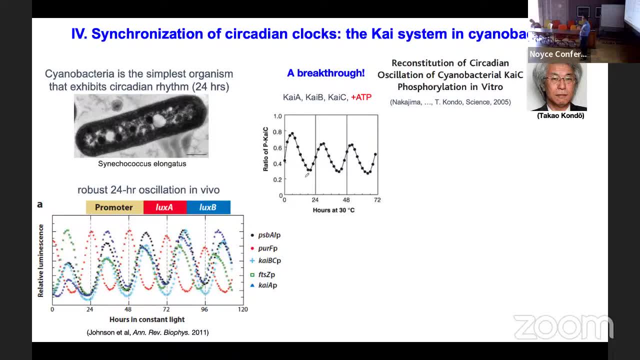 how the elegant. I mean this is probably the simplest clock you can ever, simplest autonomous clock. They are actually what people call the hourglass clock, which it can entrain to external 24 hour signal. 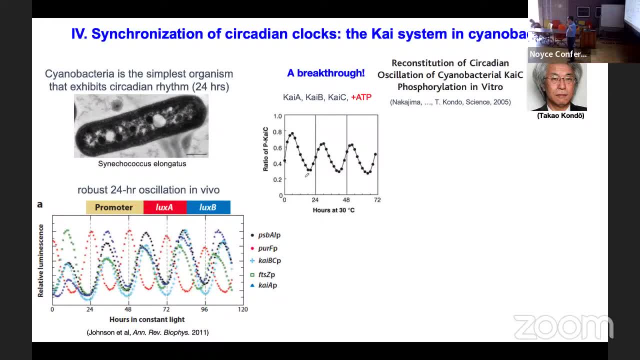 but it's only passively right. So so this is probably the simplest autonomous 24 hour clock there is in the wild, in in the whole living world And, as I said, the core component of this clock- 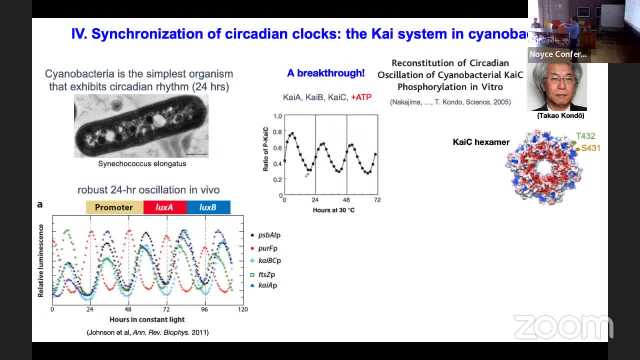 is a hexamer of chi C. chi C is the monomer molecule. it forms the hexamer, six of them On each of this monomer, chi C monomer, it has two phosphoration site. That's your tick. 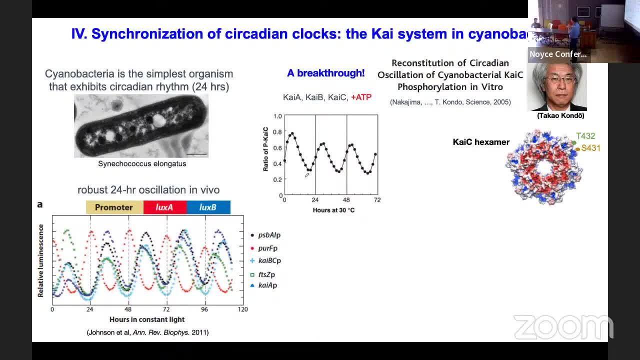 So you have 12 ticks each one. have two tick, you have two, you have six of them, you have 12 ticks, right? So that's exactly how they tell time. It tells time, for example, at 6 AM. 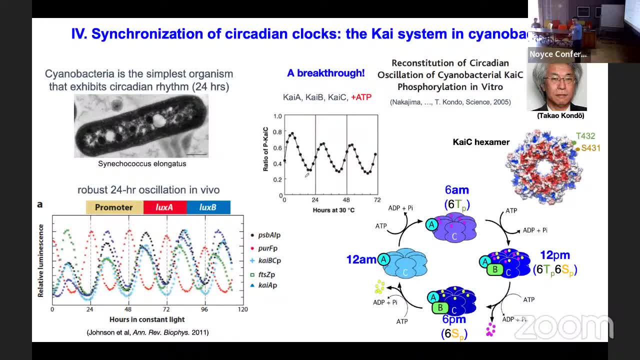 in the morning it has six T's T. so each monomer has one T and one S that can be phosphorylated. So at 6 AM it's six T. they're all phosphorylated At noon: 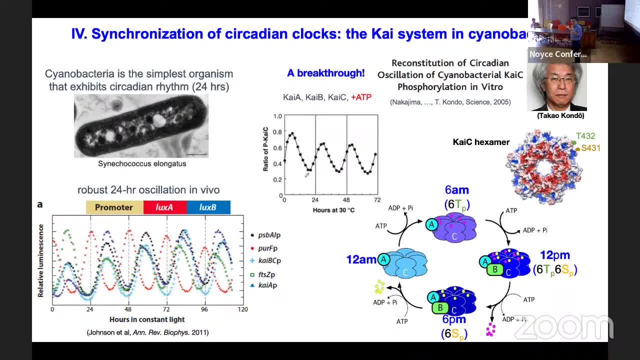 both T and S are phosphorylated. At 6 PM the six T phosphorylation are dropped off, and then six S is phosphorylated, And at at midnight right, not nothing is phosphorylated. 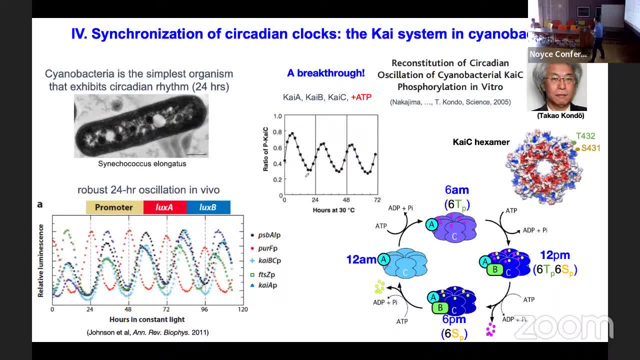 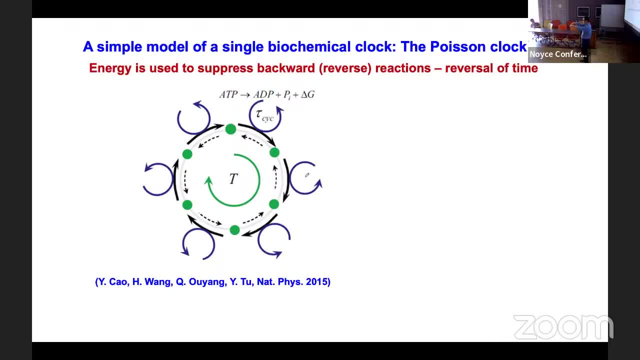 So that's how, exactly how it works, roughly speaking, right, So it's great. So how do we build a model? So we actually build model. many other people build a model for a single hexamer clock, right? 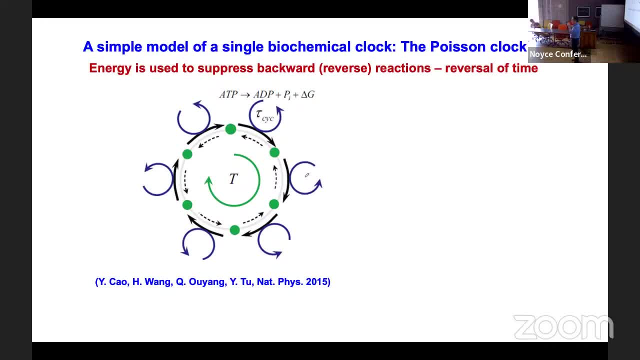 So the other component, Chi A and Chi B, are regulating the phosphorylation and dephosphorylation cycle. right, You need to be regulated, But at the energetic end of this it can be simply understand. that's why I call it. 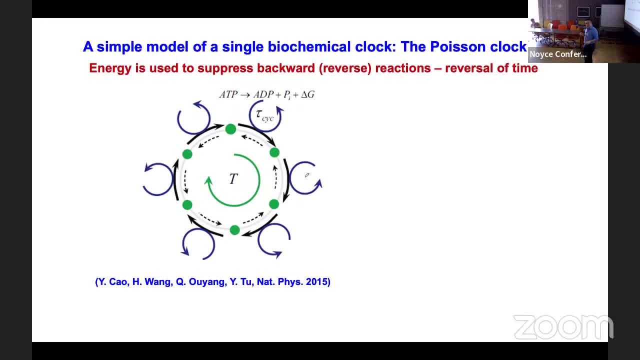 a Poisson clock. This is the representation of a single clock and it can go so, once you, the clock ticks because of phosphorylation and dephosphorylation. right, And that's other half. So basically, 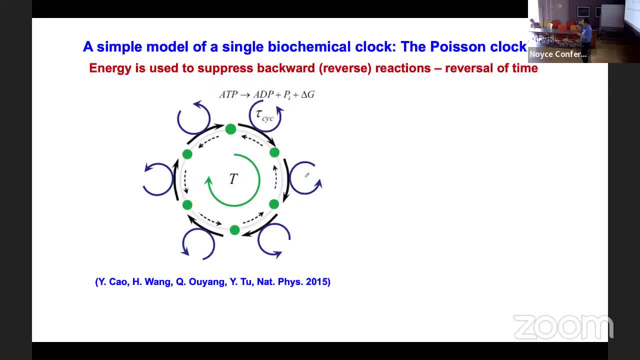 you go forward because the phosphorylation is in hand, the reaction is in hand, the thick line, thick arrow, black arrow is enhanced by it's coupled to ATP hydrolysis, so it's really enforcing the forward. 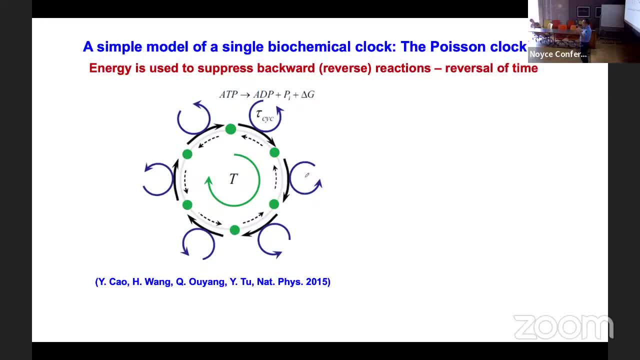 If, if it's a random walk, it's not a clock right, So you really push the forward rate much higher than the backward rate. That's how you create a single hexamer clock at the bottom of it. 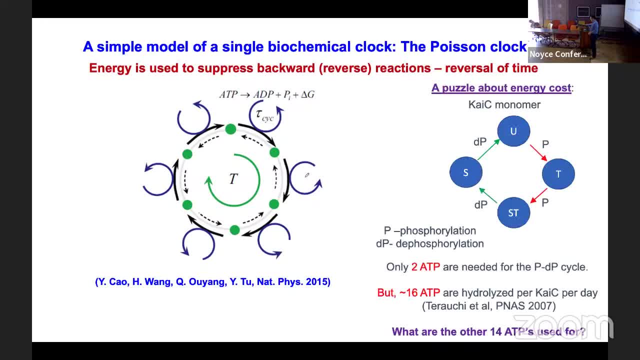 right. So this is a very nice and good and and, but then we know this cannot be the full truth. but we also know this from direct biological measurement, energetic measurement. So this picture, left hand side. 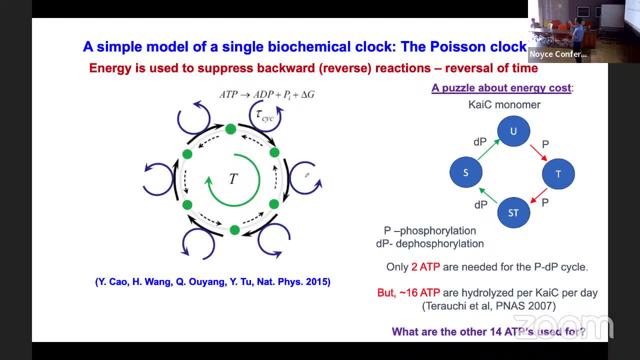 it basically says: well, okay, so each monomer as it goes through the full cycle: it goes from not phosphorylated to one phosphorylated, to two phosphorylated and and then one dephosphorylated. 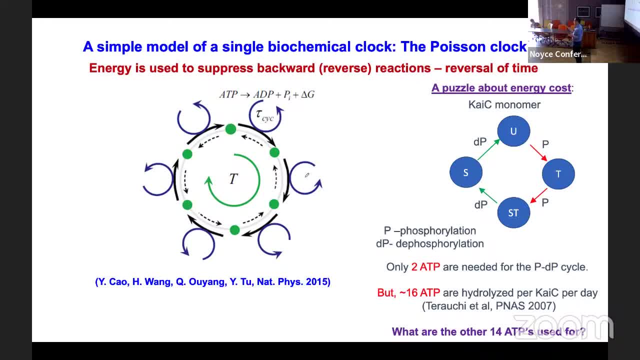 two dephosphorylated and back right Per per cycle. how much ATP does it cost? Two, right? You need one ATP to give you one phosphate group, That's. that's the minimum it takes, So it should cost you. 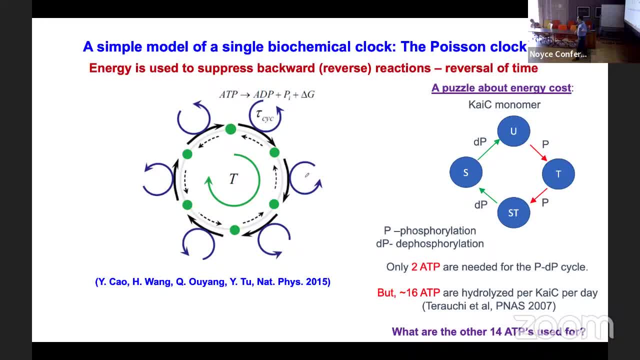 two ATP per 24 hours, But actually people actually did measure this. Yes, That's a good question. Nobody actually knows. It may be sequential, but that's a separate you know thing that people still want to do. 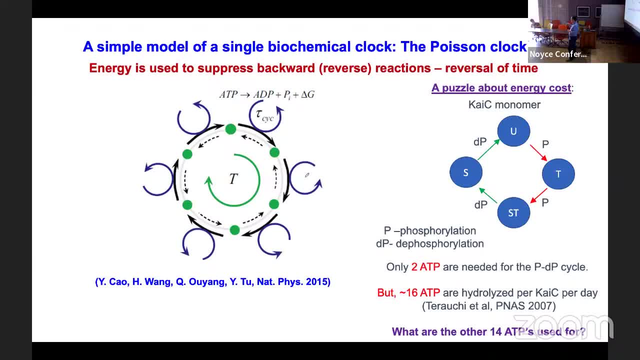 Yeah, it's, it's. and also whether Y is T phosphorylated first and then S second, what So? the sequentiality is a very big thing, because I I put this as a direction. 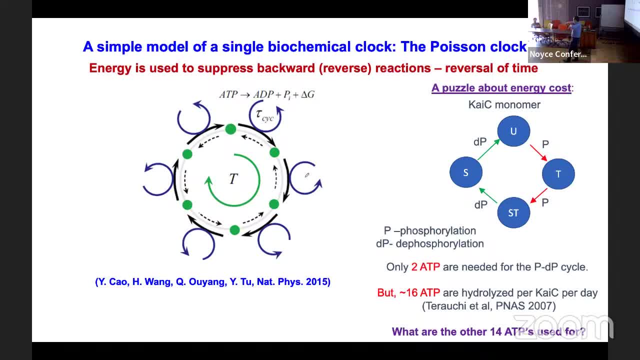 as a, as a linear curve, linear reaction chain. But it may not be. it may be a much, much more complicated network. Yeah, so back to the story of energetics. So people actually measured how much energy is dissipated. 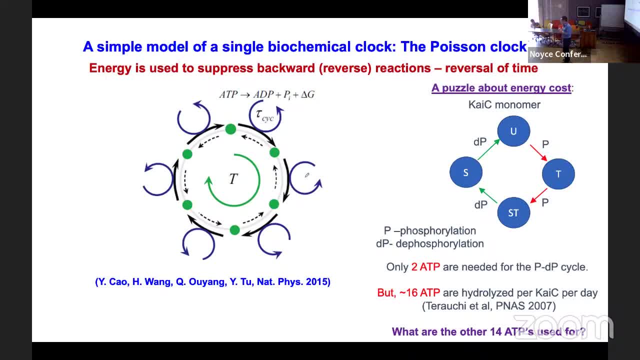 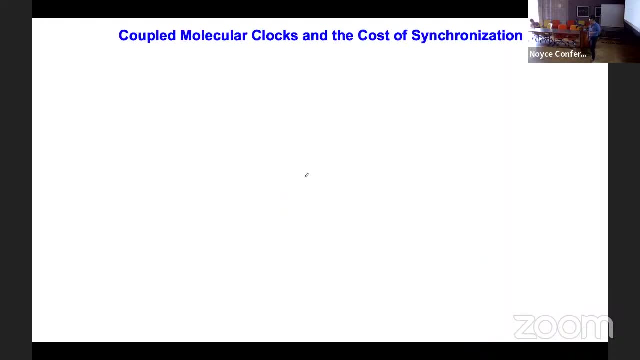 per cycle. per monomer, The number is 18.. So where did the other 16 went Right? What is it? Just wasting energy, Or doing something else more useful, Then? okay so, so now it comes to the punchline. 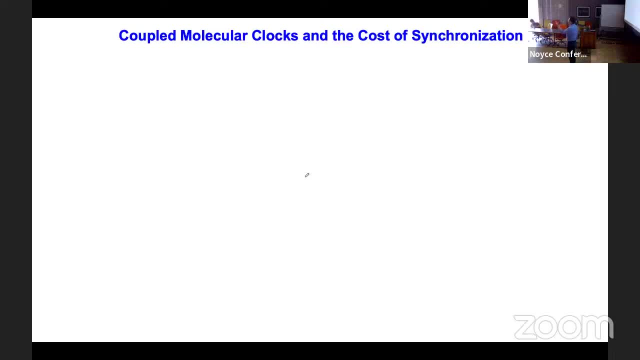 is that the cost of synchronization? So the problem with a single hexameter clock is a very nice and elegant, but it's very, very noisy, right, Even if you totally suppress the backward reaction, the dotted line. 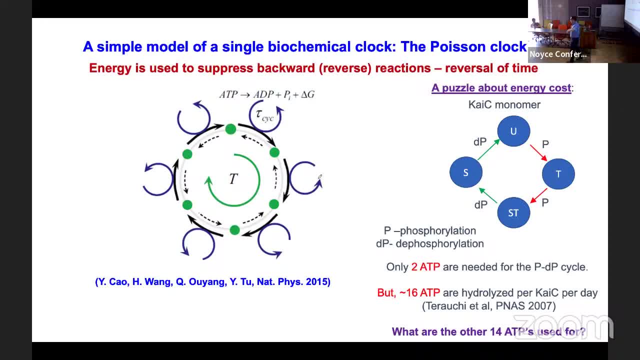 if you totally set it to zero, you're still a Poisson clock, meaning that the process of going from one from from 12 o'clock to one o'clock is still a Poissonian. It happened the duration of that transition. 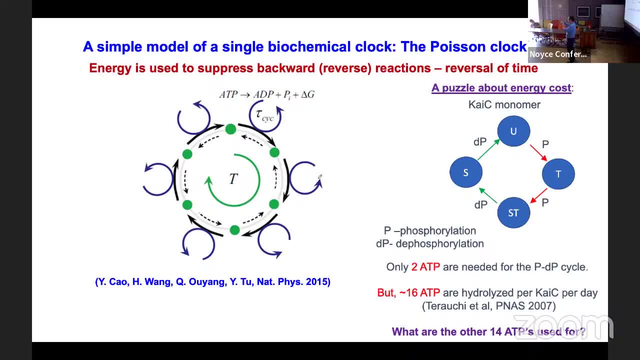 has a very broad distribution So, as a result, your 24 hour clock cycle is very imprecise. So the problem with that is that each individual clock is very. is that each individual clock if it's running by itself? 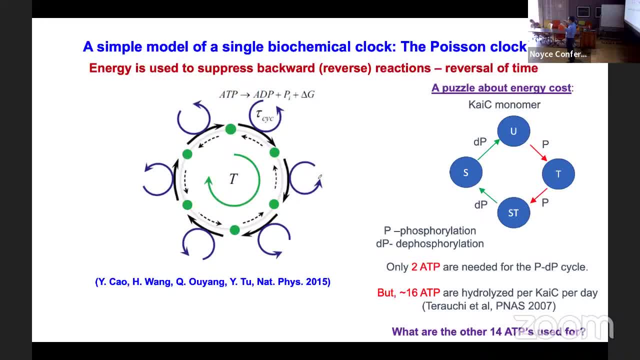 and everyone has a little bit of error, 24 hour error. if you average together, the phase decoherence will happen very quickly and you don't have a clock anymore at the population level, Right. So the fluctuation? 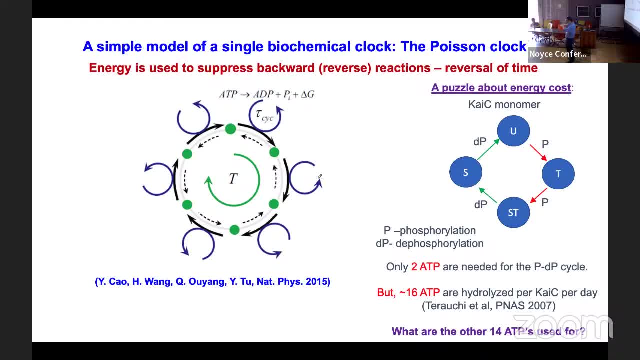 the oscillation that people measure are really the averaged population, average over across the whole population of tens of thousands of such a hexamer. So you need synchronization between them. You need synchronization going from a single. 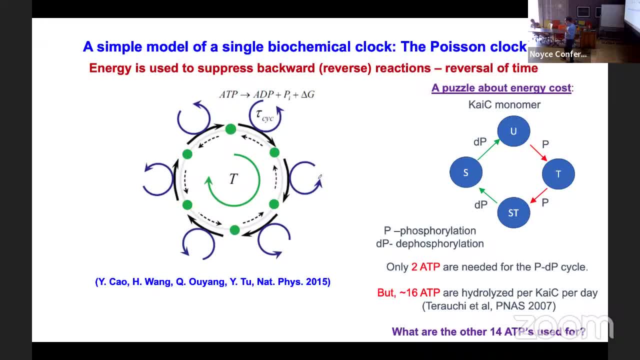 molecule clock to actually a coherent clock that can be observed macroscopically and can be used to drive actually biochemical synthesis and gene regulation. So that is the problem, general problem from the theoretical side. 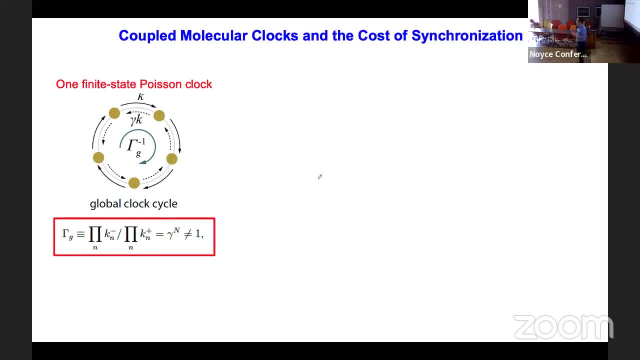 So okay, now we need to build a model to actually try to understand synchronization. We say, okay, we know how to build a model to do synchronization, but let's start from since. we're trying to understand energy cost. 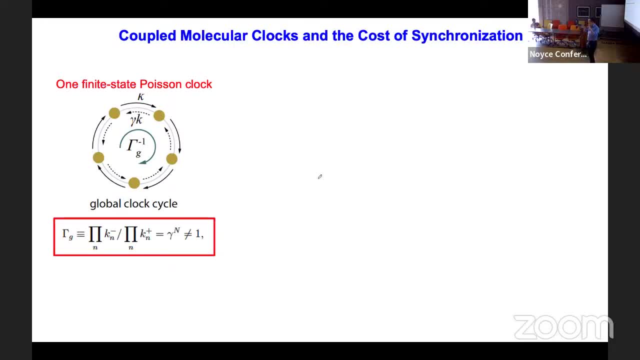 let me try to first figure out: what does energy cost come in within the framework of Terry Hill? Okay, So Terry Hill told us we should look at the reaction cycle. this is the cycle right And we should multiply. 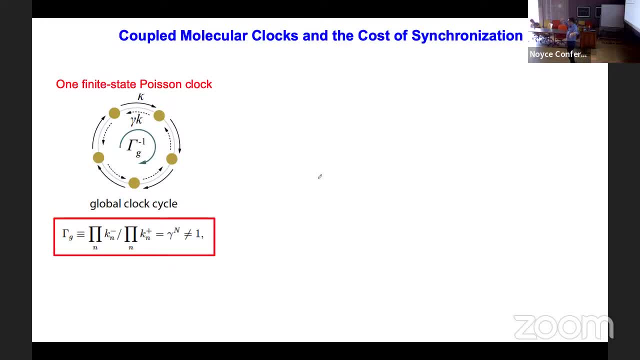 all the rate going clockwise, literally clockwise, and divide by the rate product of the rate going counterclockwise, And you get that, and you get gamma m. Gamma is a very small parameter, right, Basically suppression. 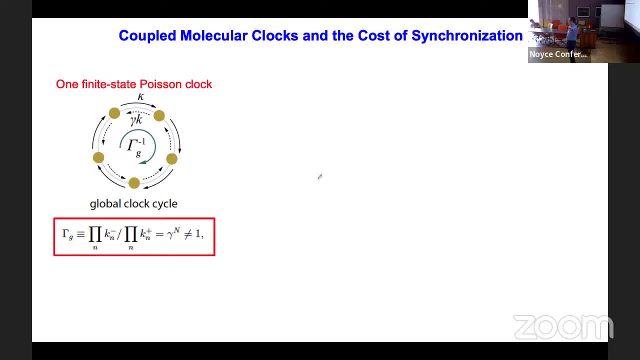 the reverse reaction. So that obviously is not equal to one. So a single clock, single molecular clock, costs you energy. That's the two ATP, that okay. So how do you allow different clock, molecular? 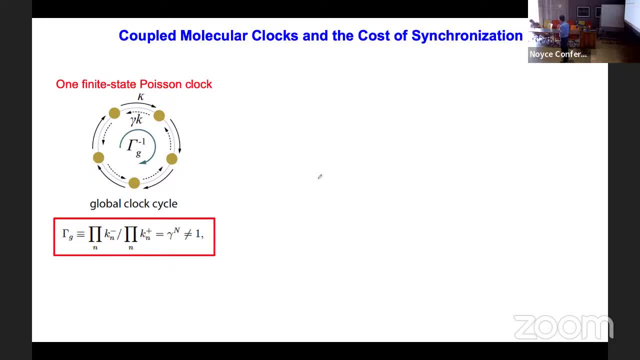 highly noisy molecular clock. to synchronize, You have to have allow them to interact with each other, right? Otherwise how are you gonna synchronize? So you allow them to communicate with each other? And, as you know, 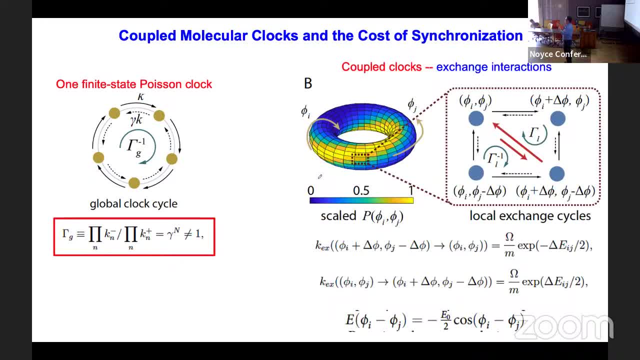 from physics point of view, this is actually not that hard. You just allow them to exchange right. So you have, because phase is really just the number of molecule, number of phosphoration site, If you allow two clock. 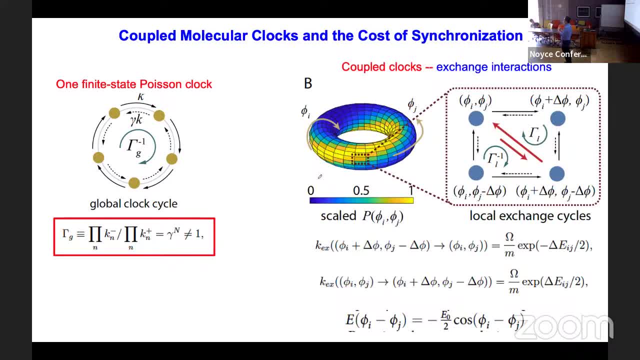 to exchange the monomers, for example right, And you can introduce interaction between different clocks. So this can be is presented by two clock, two such molecular clock represented by the phase in the torus. 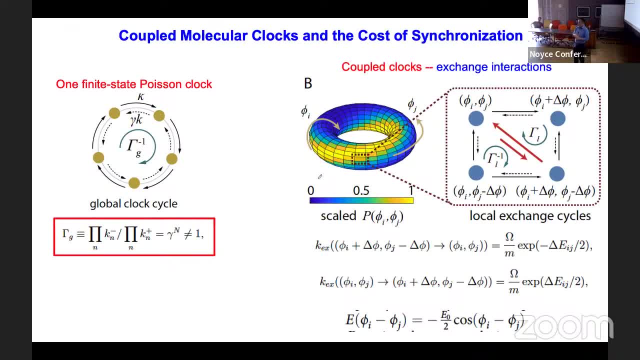 And we introduce what we call the exchange interaction. So other than the big cycle, so you have a doughnut, you can go a cycle along one side and the other side- But you also allow interaction between 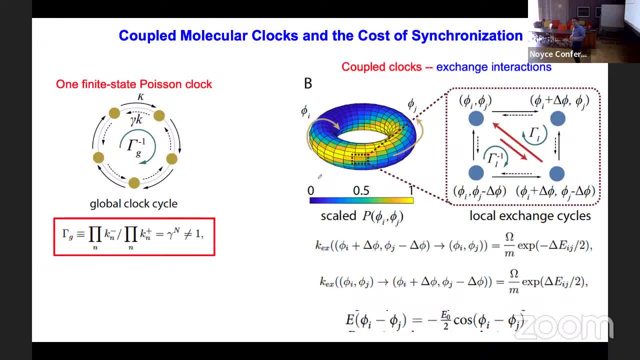 the diagonal, I did two. the two red line correspond what we call the interaction. So I'll tell you later what what does represent. But mathematically this is the kind of interaction we we introduce. 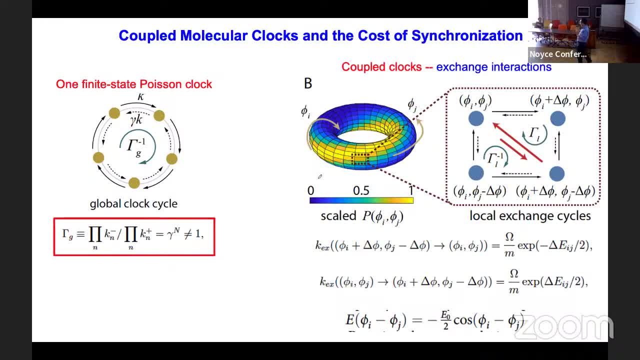 In physics that correspond to interaction, Basically exchange interaction between two oscillator. So the interaction, because it's a chemical interaction, you have to introduce a frequency or the rate. That's one thing, And the intensity. 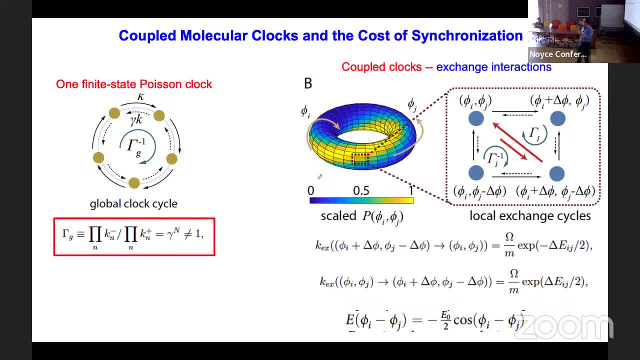 how strong the interaction is. So so omega, capital omega, tells you the the frequency of that interaction, And delta E or E zero correspond to how strong this interaction is. So introduce that. 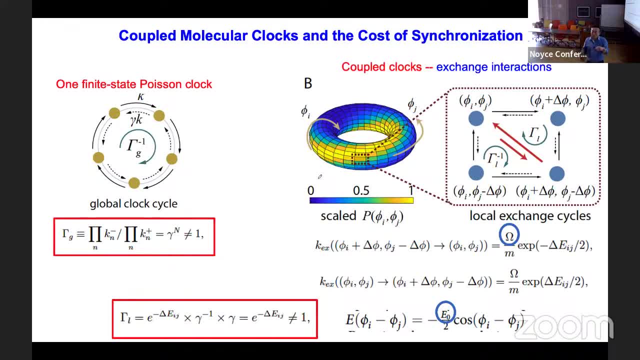 And what? what do you do with such a model? So omega and E zero, And then you, other than this big cycle, you actually created also local cycle, Right? And if you look around the local cycle, 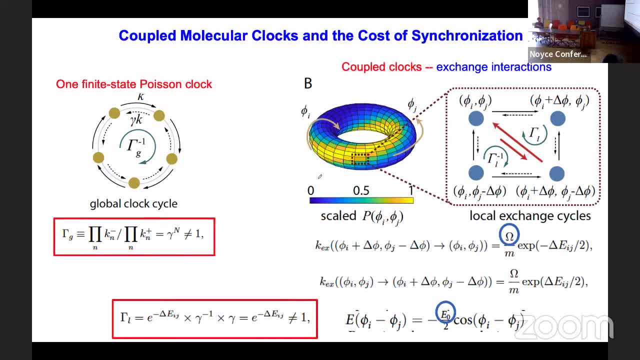 it also the gamma capital, gamma L local. it also not equal to one, Because you have the exchange interaction, When E zero is not zero, So that also causes energy. In other words, by introducing the exchange interaction, 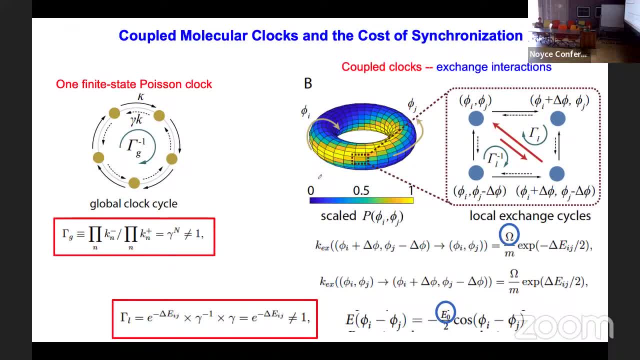 also, you have to pay for it. Right, Of course, that this interaction is synchronization. Therefore, that's how we relate the cost versus the performance. The performance in this case is synchronization. Technically, you actually 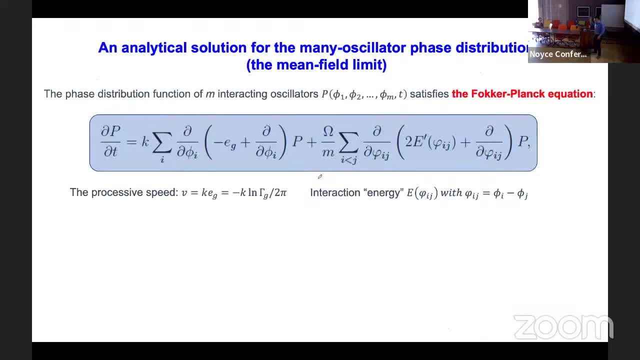 it turns out. this is actually very nice At the mean field level if you allow every yes. So in the first, like everything is happening still in the hexamer right. So is it like the? 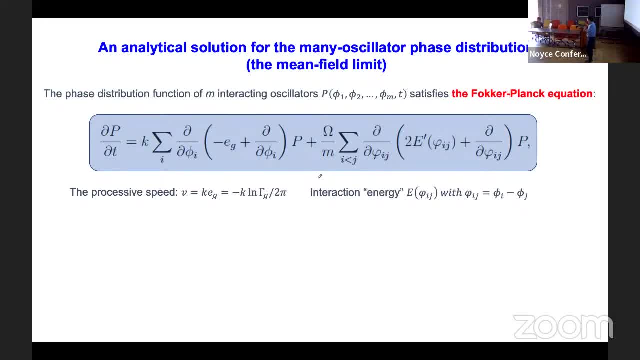 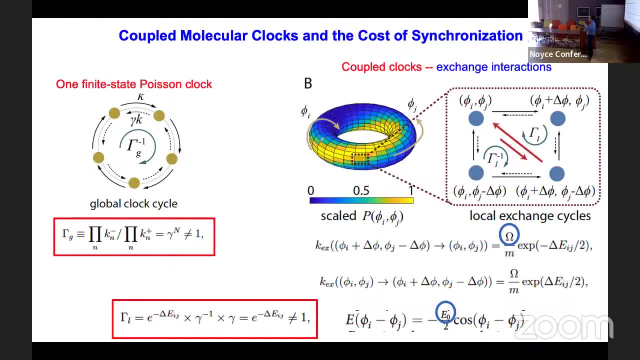 No, this is happening between two hexamer, Between two hexamer, So is it kind of a conformational changes that's? Oh, I'll get to that. What, what, what causes this interaction? Can you say something about this? 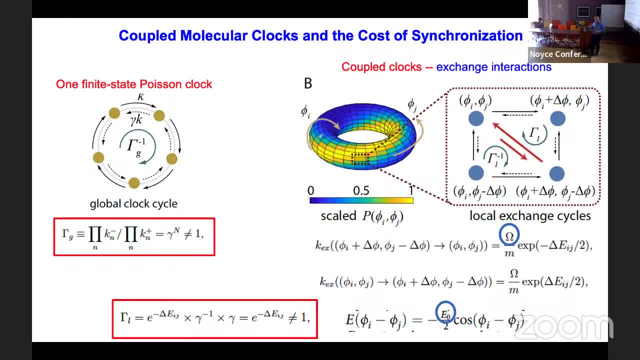 delta EIJ, Because I'm just surprised that it would have that form. Oh, delta EIJ. okay, this particular form says that it prefers the two phases to be the same. In other words, if you but this: 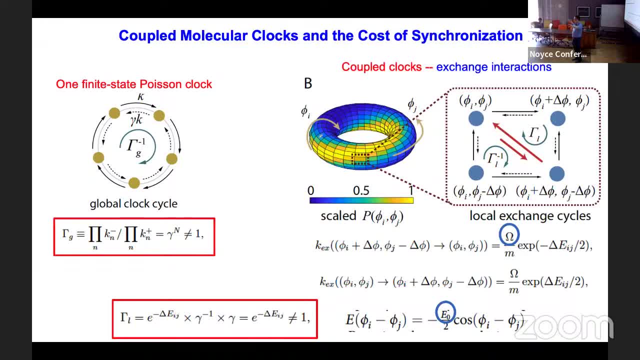 that doesn't have to be the case, But in this particular form we say it basically is a ferromagnetic coupling. Okay, But you're right, There's no reason to say there's a ferromagnetic coupling. 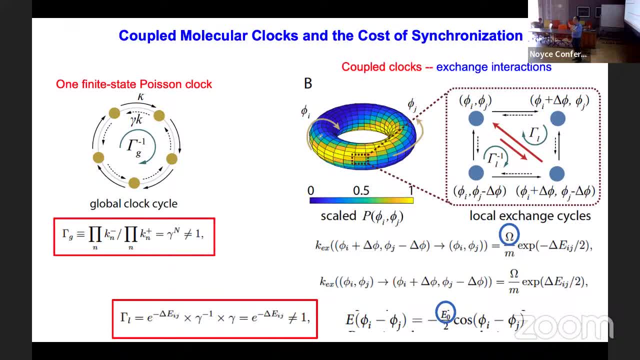 So we have done. later on I'll show you done simulation where it's just the random shovel, That's enough, because entropic effect. So if you have two clock, one is at one o'clock. 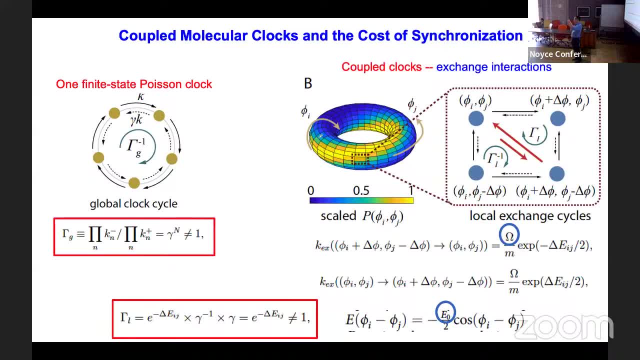 another one is at the four o'clock. the likelihood of being in two and three is better than the likelihood of being 12 and five. Okay, so, so. yeah, that's a good question, But here. 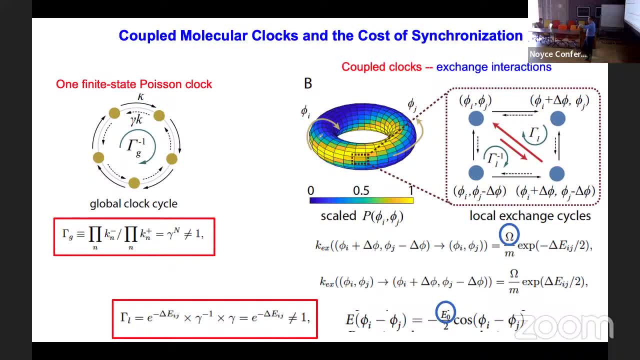 we just theoretically. we treat this problem like this. As you see later on, we actually have a more realistic model of the hexamer, based on realistic mechanism, molecular mechanism to do the. but this is for theoretical study. 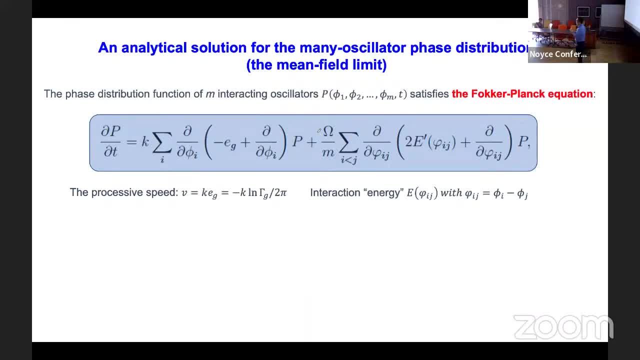 right, So we wanna. so actually, this model, if you allow in the mean field sense, if you allow every pair to interact with equal probability, that's definition of not crazy. because, given the fact that 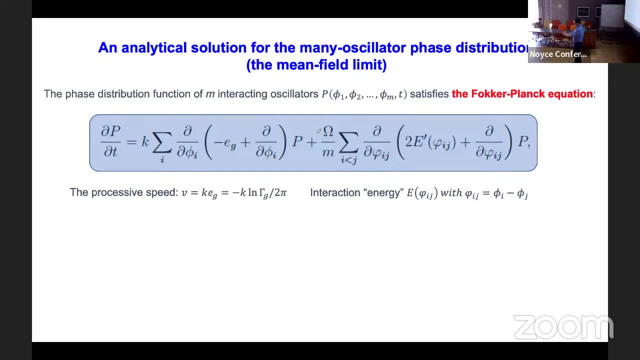 diffusion. this is in a suit. in a suit, imagine, you have what is hexamer. they interact with each other, by collision, let's say, and diffusion is fast enough. we're talking about hours, right? So 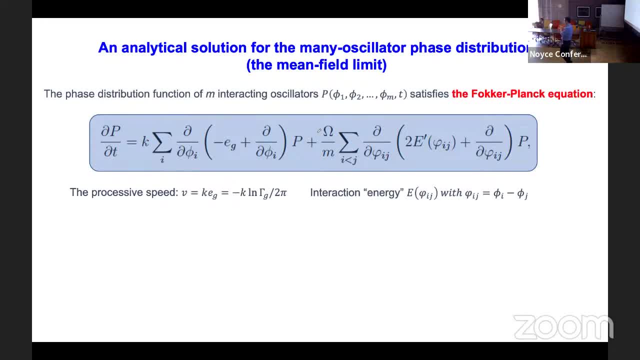 every pair is gonna see each other multiple times over the period of time that relevant for the circadian clock. So to assuming this is the mean field is actually not crazy. So we actually can solve this. 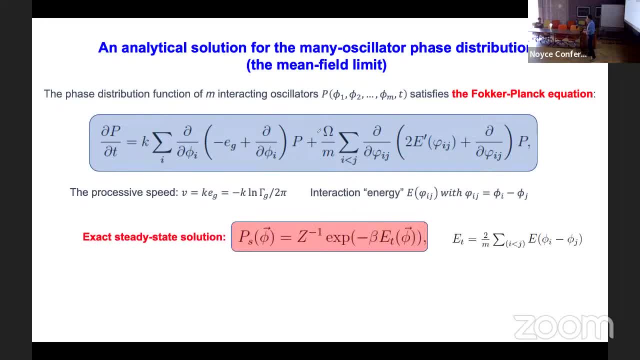 coupled, this solution is actually extremely simple. It actually all amounts to have the same Boltzmann form, except the beta is not one over KT. one over KT here, by the way, is one okay. 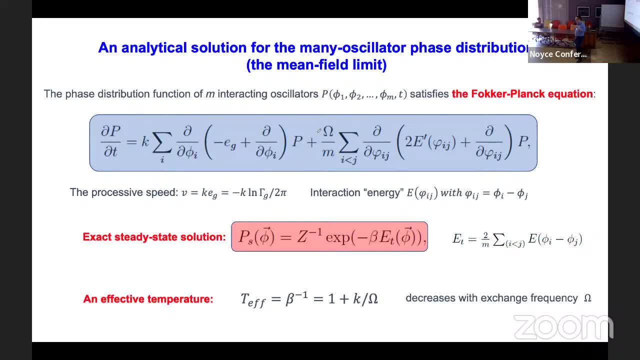 we set the thermal temperature to be one is actually the effective temperature is one plus K over omega capital. omega K is the natural frequency of the clock itself. omega is the interaction frequency, In other words, 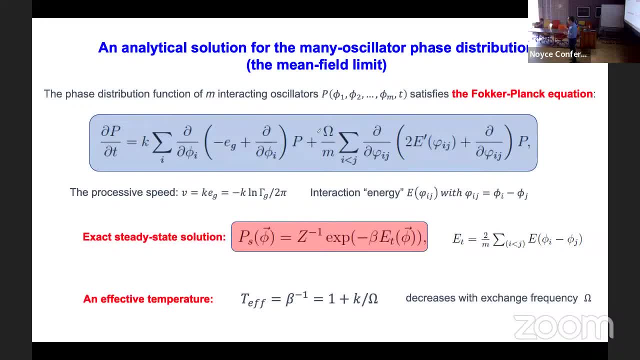 it lowers the temperature by enhanced, by increased interaction. Lower temperature leads to order, right as we know. Higher temperature leads to disorder. So if omega equals zero, this effective temperature is actually infinite, which means that 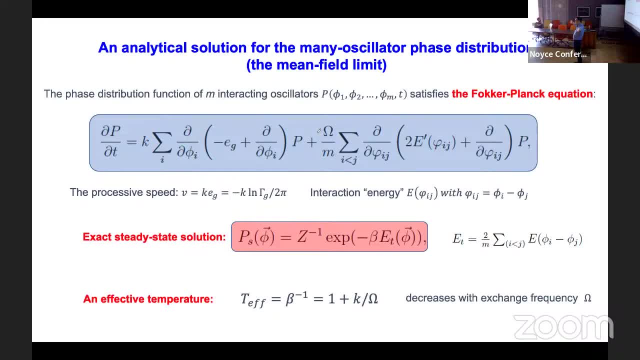 all the phases are equally probable. That's not a clock, it's just you have no concentration fluctuation. probably a fluctuation, But when omega. but omega has to be large enough to drive T effective. 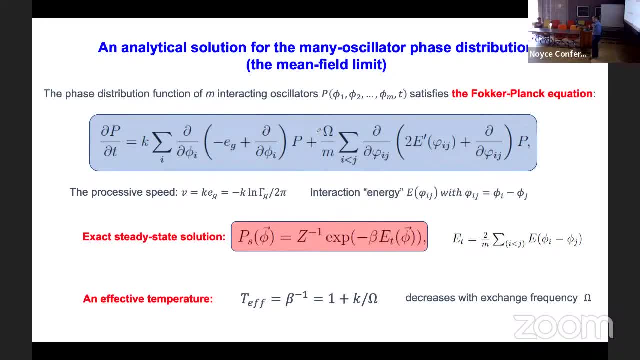 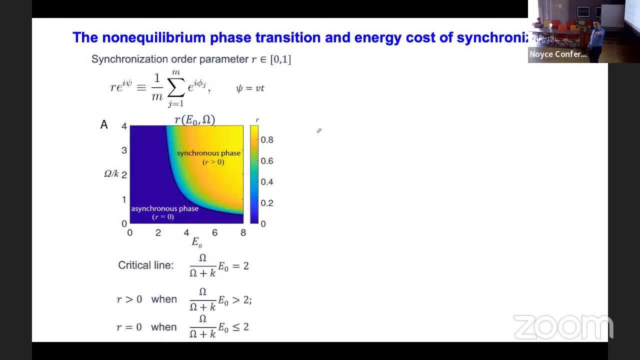 to lower than the critical temperature. We actually also know the critical temperature from equilibrium statistical physics. So anyway, so we actually can compute this critical line which correspond to this formula. And you plot it and did agree. 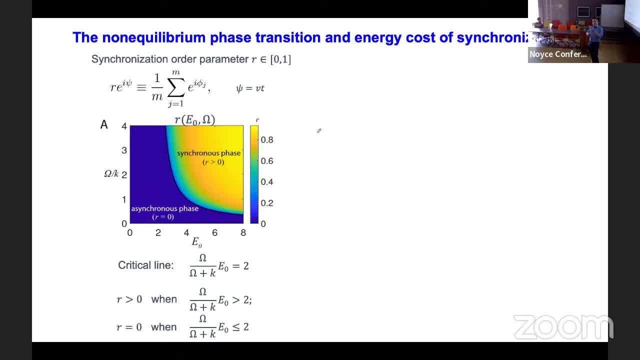 with the simulation very nicely, as it should be, But you see, there's a transition right in this dry exchange interaction space. Remember, the exchange interaction is characterized by two things. One is omega. 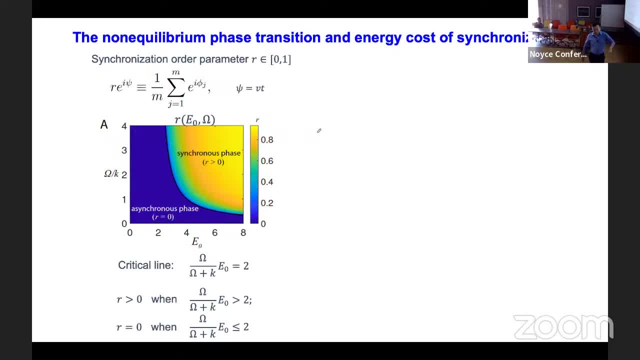 The other one is how strong it is Right. so in this phase diagram you have the frequency of exchange and strength of exchange And in this part, if you have stronger and more frequent interaction, you will. 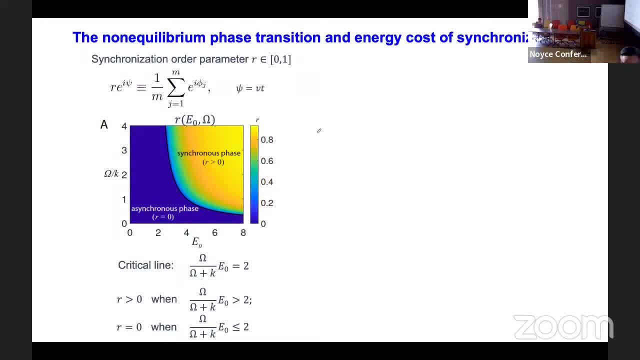 lead to a synchronized phase, Whereas if you don't have any interaction here, then you are a synchronized phase. So you need this exchange interaction and also have to be strong enough. Okay, How many times? 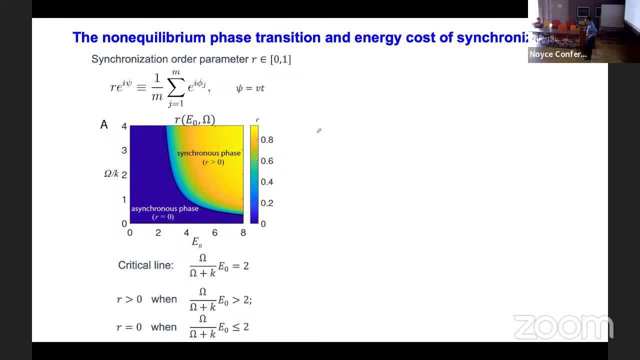 I see are there in each. I am there. I think the number I get is is tens of thousands, Tens of thousands. But it also also itself is also late with time Because it's controlled. 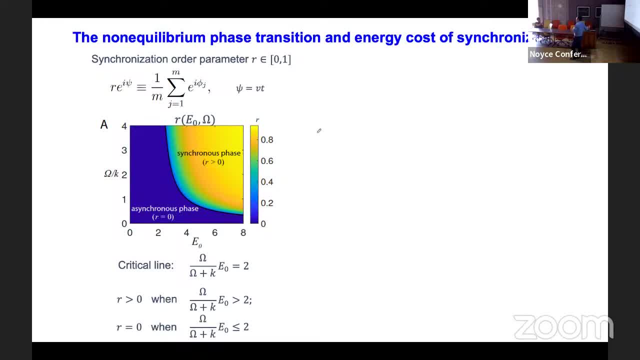 by the gene expression, which is then controlled by the, the, the clock itself, But the, the, the average is about tens of thousands. And then do you see evidence of phase separation, with, with, with these C clusters. 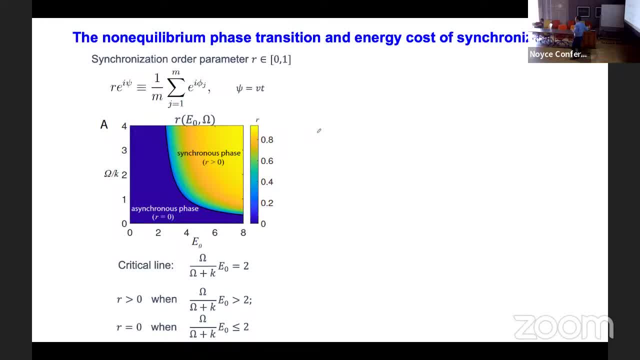 within, And is there any technical appearances of clusters there? No, You're talking about in vivo. Yeah, Uh, not, not that I know of, not that I know of. I wonder if anybody's looked. 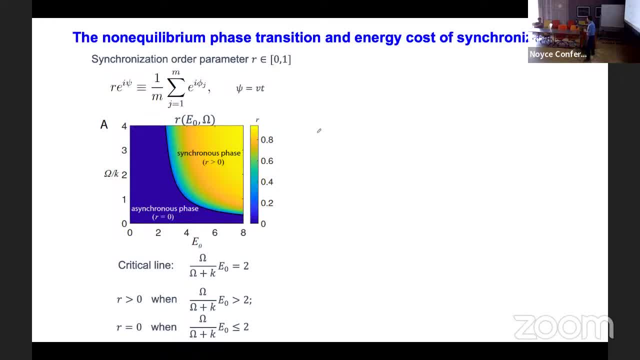 Uh, that I have no idea. Yeah, that's a good question. All right, So we can so. so this is on the behavior, this is on the functional side. this is all about function, omega and E0.. 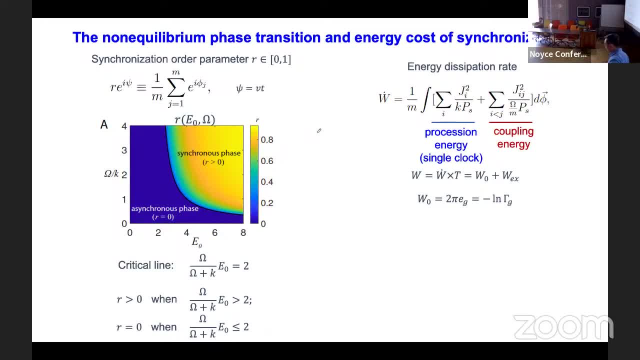 Dissipation of course also depends on omega and E0.. So we can also compute the dissipation. And also not only that, we can actually separate the dissipation, the energy cost, into the part that drives single clock and the part that drives the synchronization, the exchange. 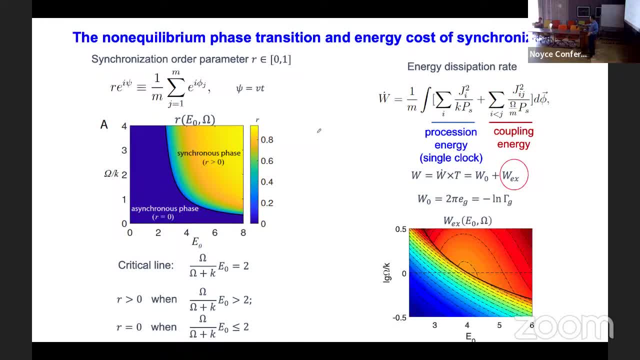 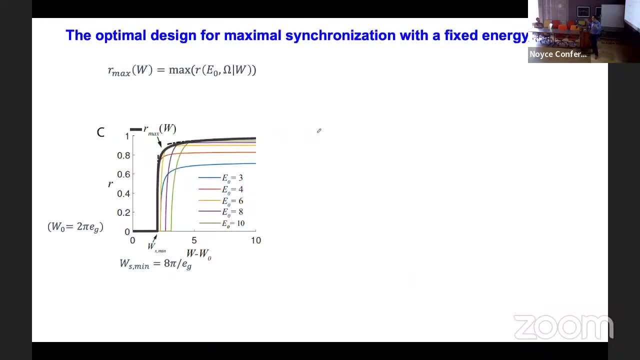 interaction, which is the red part, coupling energy. So we can actually do that for the whole parameter space And we actually can get to what looks like a critical phenomena right. So basically, on the y-axis, here you have the order: synchronization order. 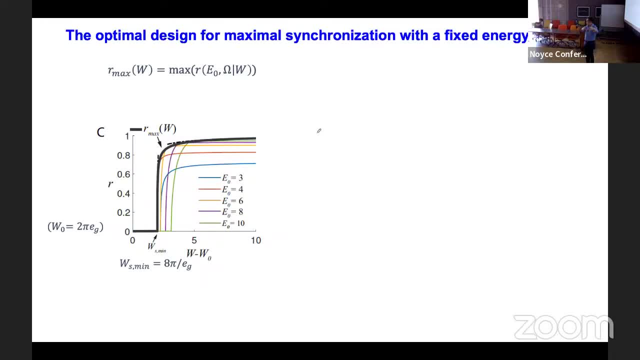 On the horizontal axis you have the energy cost. This diagram is supposed to tell you that it costs minimum amount of energy for you to synchronize, Because before that you have no synchronization. r equals 0. And after some critical number it goes up. 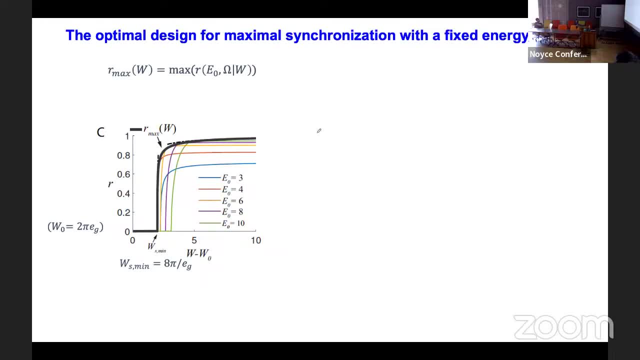 And it goes up pretty quickly and then saturates. This is the solid lines envelope for different values of E0.. So actually, not only you can get that, and this result not only can tell you this, but it also tells you that. I won't go into the detail. 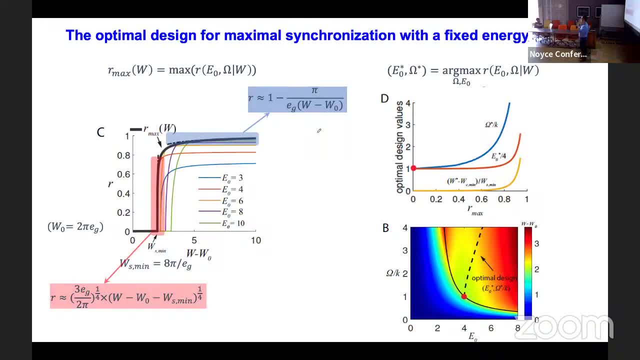 that, in fact, you actually can think about an optimum design. What do I mean by that? What I mean is that the energy dissipation depends on both the frequency of interaction and the strength of interaction. right? So if I give you a fixed amount of energy, which? 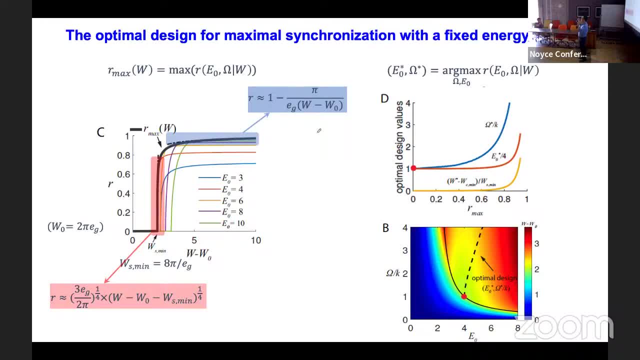 means that I have a constraint for omega and E0, what will be the optimal order r you can create right, So that corresponds to a particular line which is represented by the dotted line. This is the optimum design line. This will be the best you can do with a fixed amount of energy. 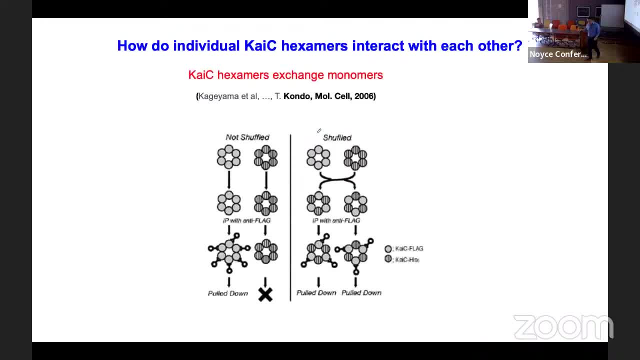 All right, so OK. so back to biology. So I tell you about the mathematical construct of how do you impose this exchange interaction. Does reality really happen this way? Actually, it turns out, indeed, it does. This is actually Actually. it corresponds to another sort of unrelated piece. 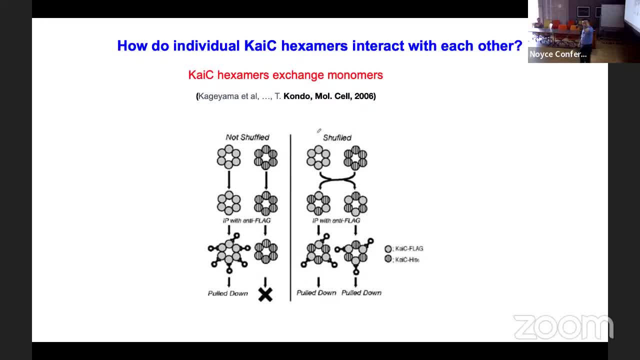 of experimental data. So in 2006,, also in Kondo's group, what they did is that they have two batches of chi c hexamer solution And one they label In one batch, one soup. it labels with this tag: 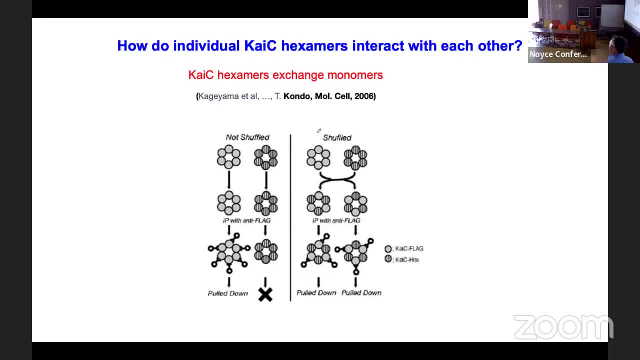 this thing right Now and then they mix it right. If they all stay by themselves Without exchange, then only half of it would be pulled down. They have to pull down. This can be pulled down by some immune agent. 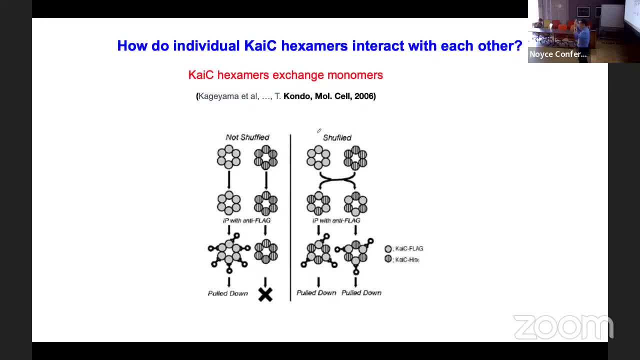 So when they do the pull down, what they find is all the hexamer is pulled down, meaning that they have exchanged partner, They have exchanged monomer, So exchange monomer, So exchange monomer is exactly monomer shoveling right. 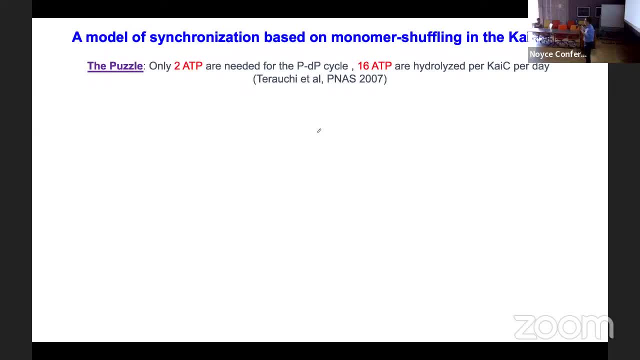 So OK, so the puzzle. Now We can sort of try to answer the puzzle. going back to our puzzle, Where does the other 16 ATP are hydrolyzed? So to answer that, we actually built a model based on the monomer shoveling. 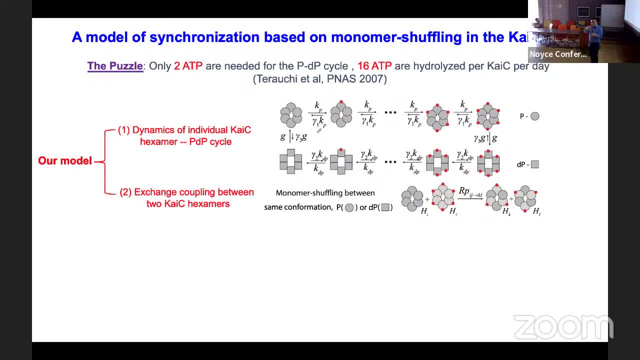 So what happened is that you have the dynamics of individual chi, c, hexamer going through the phosphorylation- dephosphorylation cycle. There's a lot of bells and whistles built into that model. I don't want to bore you with that. 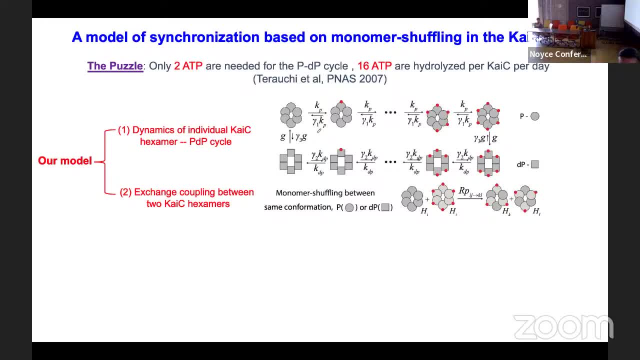 But the critical part is that we're adding the exchange coupling between two hexamer- any two hexamer. So this is the same thing as shown illustratively like this, So they actually can go and exchange with some frequency. Now we're called the frequency R, capital R. 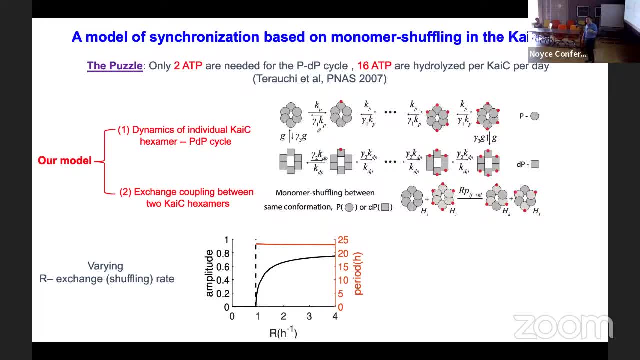 So pay attention to the capital R. So what we found is that indeed, the amplitude of the oscillation of the whole average population over all the hexamer we simulated actually only becomes non-zero. only start to have a real, coherent oscillation if your exchange rate is bigger than every more than. 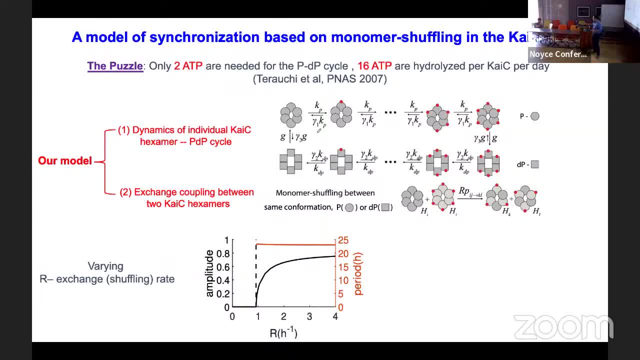 more than one every hour. OK. And once it becomes ordered, the frequency- actually the period of the oscillation- doesn't really change. So it's pretty robust against changes in R, But you have to be here for the amplitude to be actually finite. 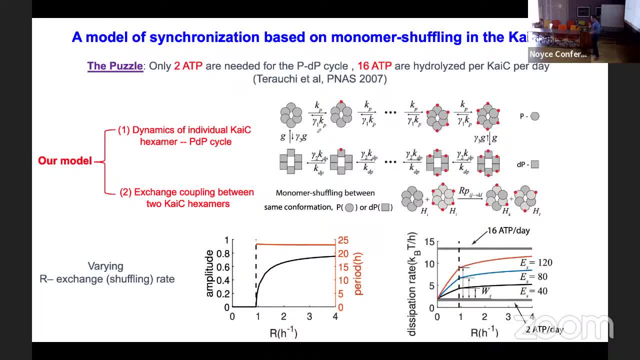 Now, on the other side of the coin, which is the cost, we can also compute the cost And indeed we see that, assuming different interaction strands the es you actually can get. this is the two ATP that you started with. 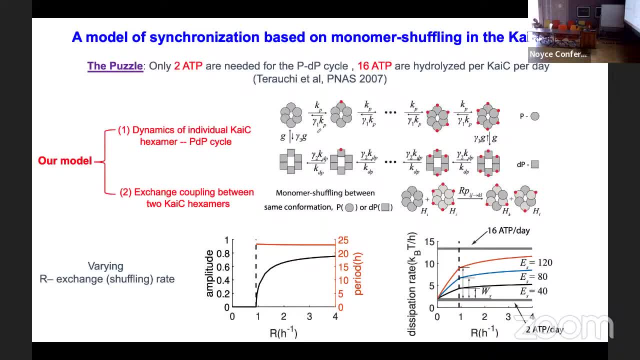 You actually depending on R. R increases with R And it actually can get closer to the 16. In other words, additional energy cost is probably needed for driving, whatever mechanism you have for the synchronization of individual clocks. Yeah, Is it better to exchange in an unphosphorylated molecule? 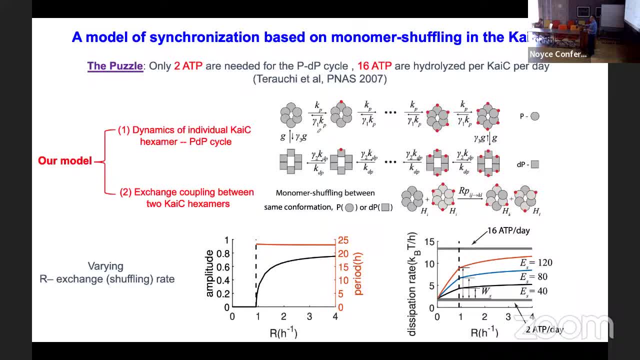 rather than to dephosphorylate an existing one. Yeah, that's a good. so we are still working on this model. This model assumed that both the dephosphorylated and phosphorylated can exchange between them. any hexamer pick can exchange. 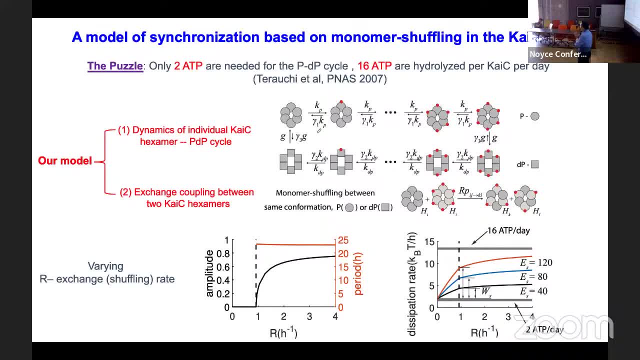 Experimentally it was found it only predominantly happened in the dephosphorylation phase. So this is the future work that we're working on. We have a good idea now, because what I'm telling you only half of the story. 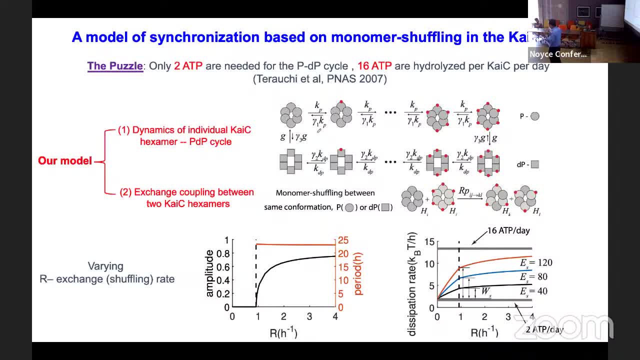 There's another mechanism people believe is relevant for synchronization is the weighting mechanism. In other words, if you're in the phosphorylation part of the cycle, if you're more advanced, there's a. chi-A is in short supply. Chi-A actually helps you, help the phosphorylation phase. 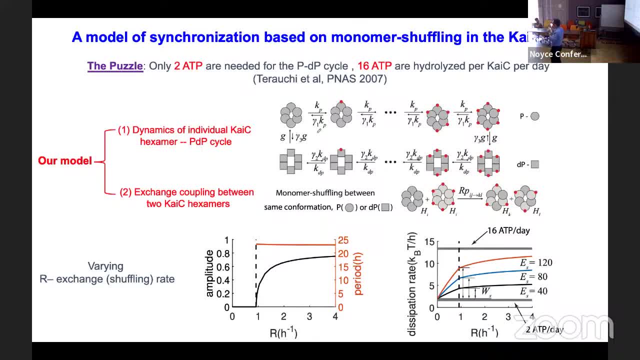 So chi-A has a higher binding affinity to the one that lagging, as compared to the one that is more advanced. So, in other words, the phosphorylation, the clock that runs a little faster. we actually wait because it run out of the whatever, not fuel. 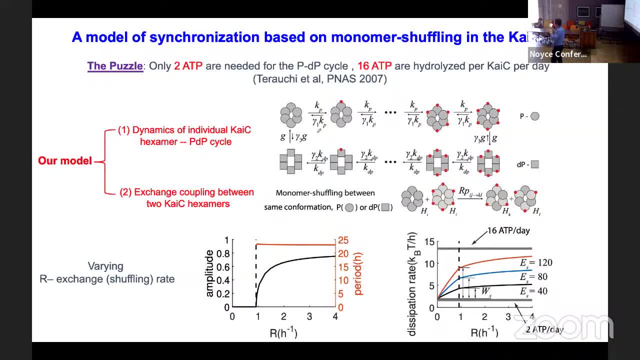 one of the enzyme of chi. So chi-A, which is the enzyme for phosphorylation, actually is nucleotide exchange enzyme. actually prefers to bind with lower phosphorylated chi-C hexamer. So that was another mechanism. But that mechanism only works. you see what I described. 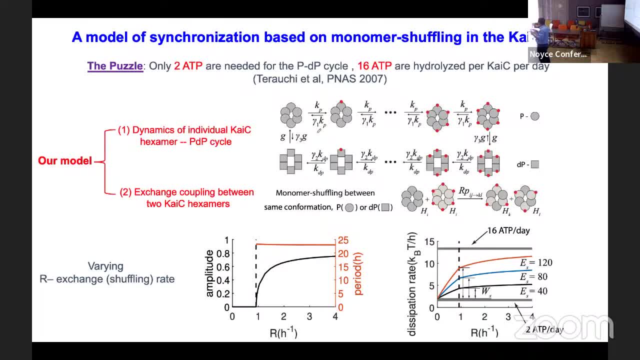 only works in the phosphorylation phase. So this mechanism comes to help. That mechanism is not enough to synchronize the whole period, because but then this mechanism helps at the dephosphorylation side, because then you can use a different mechanism. 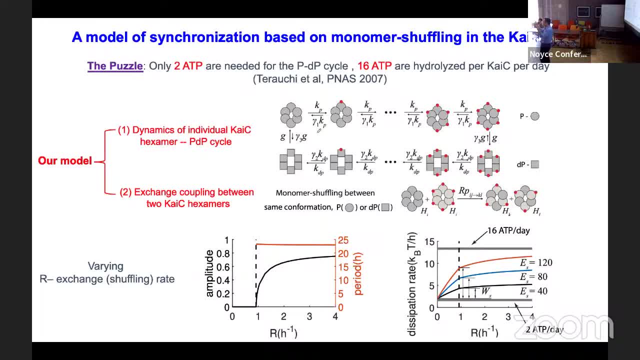 So there's two mechanisms can actually work seamlessly together, one in the phosphorylation phase, the other one in the dephosphorylation phase. So that's the current status, which is not talking about here. I'm focused on just monomer exchange. 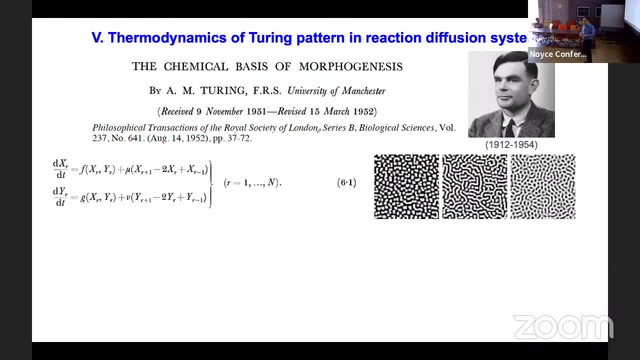 All right, so I probably don't have time. I'm just giving you. so I told you about ordering time. right? Ordering time is actually tricky business. You have to do it in the molecular environment because the high a lot of noise. 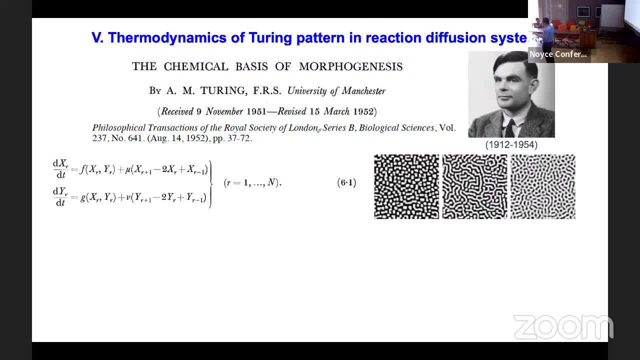 Even you have this wonderful hexamer which can have the oscillation, but because the noise will kill it if you just simply average over a large population, You have to allow them to interact with each other, which causes energy. Now the same thing goes to here, if you think about it. 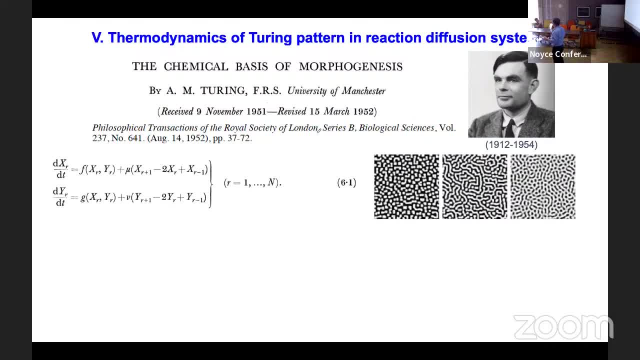 about spatial ordering. right? How does spatial order happen? The neighbor has to talk to each other, because why do I have to be You? think about a stripe. You are a low concentration and then next one have high concentration, And after some period of time you have to repeat it again. 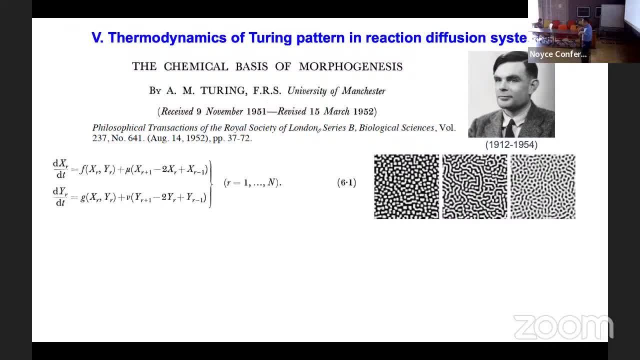 So in space, if you want to order in space, you also cost energy to do that. because just by pure diffusion is against it, right? Diffusion says you have to be uniform. So how does energy is being used to actually overcome diffusion? 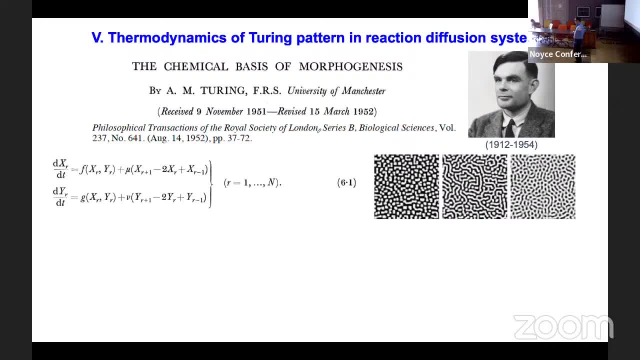 to actually give rise to spatial order. So we end up studying: What's a spatial order? Well, what is it actually? It's a superimposed, And it's just in the space-time-time space as I'm presenting. I mean, it's the space-time-time. 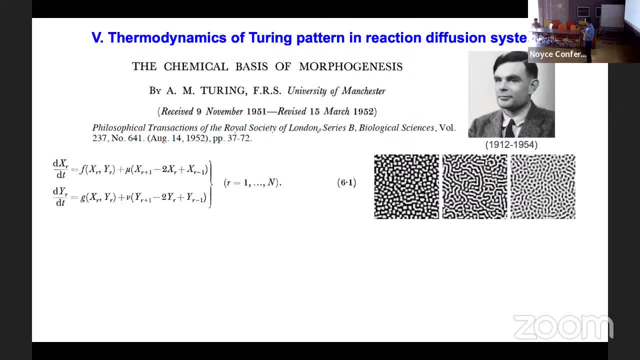 So the space-time, space-time, that's what's called the dimensional space. It's the space-time space. So here it's a superimposed energy and it's superimposed energy, But it's not always the same, Because it's just the energy that we put together. 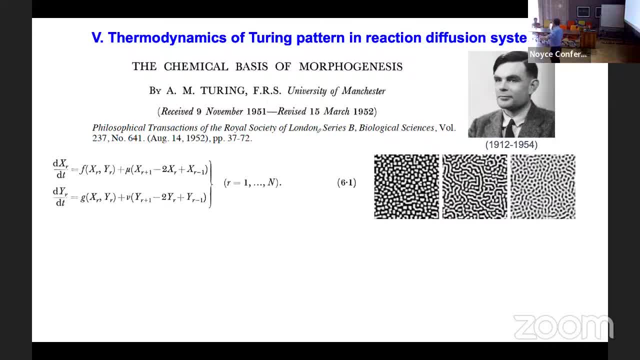 So these are some examples, So some of the real problems that I have to make. So, for me, I am looking at this, I'm looking at it, But anyway. so the equation is very simple, right? You have two coupled equation, x and y. 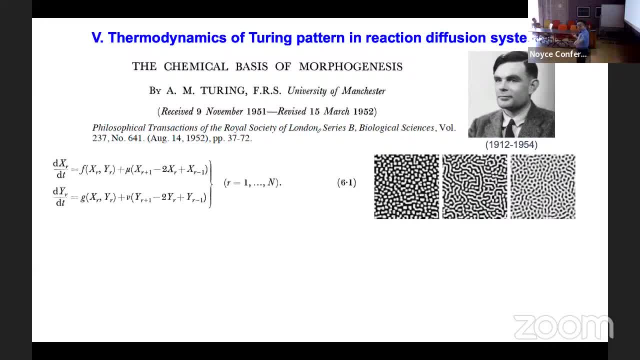 f and g are nonlinear function. And then you throw in some diffusion. So the latter part of the equation, the diffusion, with diffusion, constant mu and nu for the two species x and y. And what Turing's great insight is that, yes, 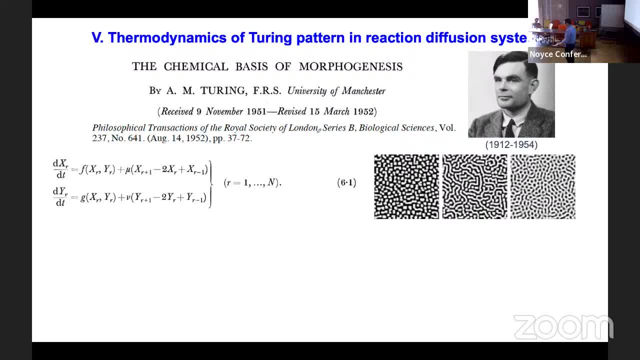 the diffusion. try to even out the pattern right. There's no diffusion against any undulation of the concentration. But if the diffusion, if the reaction parameter of the reaction, the reaction rate and so on, the driving is strong enough that you actually 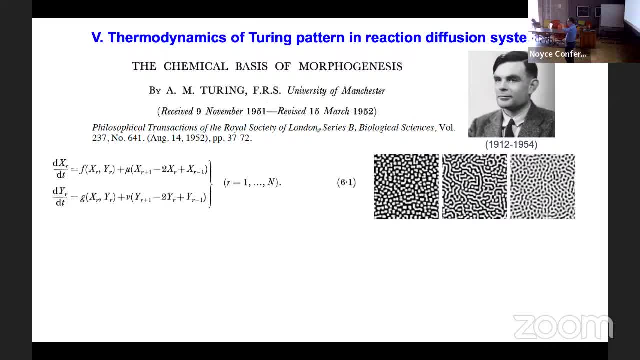 can overcome that And, as a result, you can get Turing pattern. So the homogeneous state is it becomes unstable through the Turing stability And, as a result, if you're in the unstable regime, then the system will go to a system or go to a pattern, like shown right hand side. 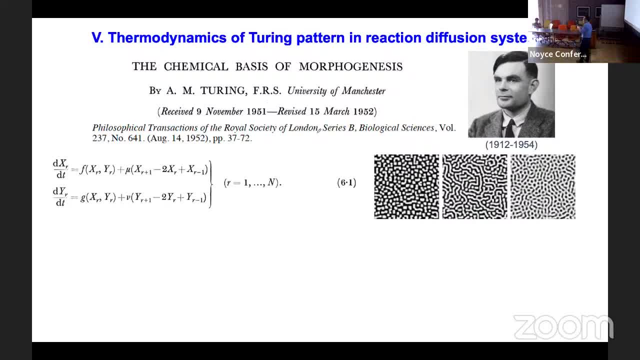 have this very regular pattern, Not very regular. have regular pattern with a very visible period. spatial ordering: OK. so what does that have anything to do with energy? Actually, my friend always tell I mean, there's a friend who is very interested in the system. 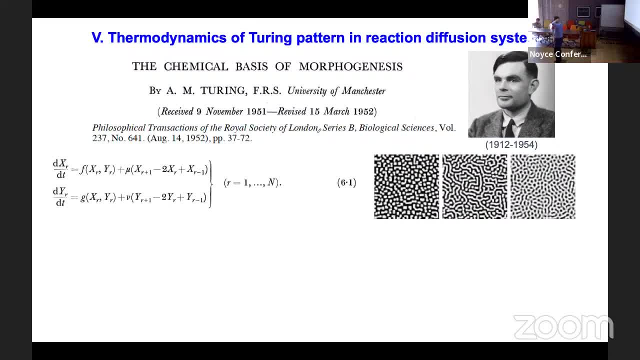 in biological system. He says: well, Turing's paper is often cited but never read. So I think it's very true, because I for one didn't only read the first part. I didn't go to the second part. So I found reading because of my interest in thermodynamics. 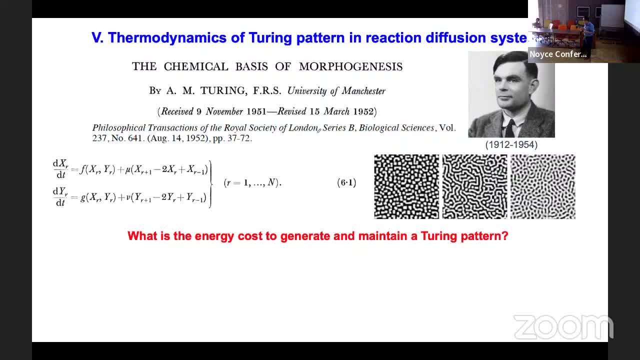 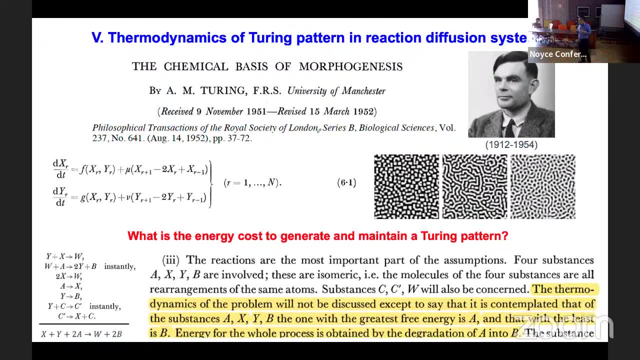 So we are interested in this question: What is energy cost to generate and then maintain a Turing pattern ordering space? Sure enough, if you look carefully in section 3 on page whatever 25, Turing had this very encryptive. I mean, he's a code breaker. 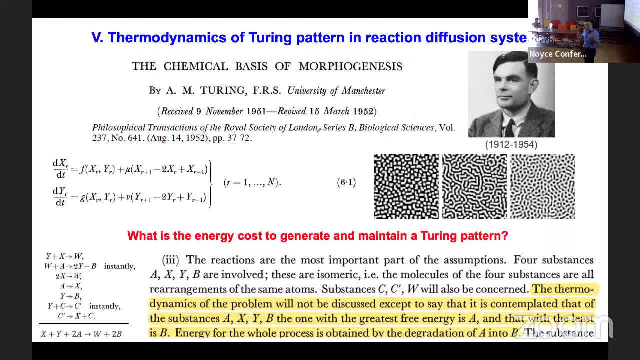 right, He has this code name. He has this code name. He has this code name. But this is actually pretty cool. I mean to me now it was pretty clear. He says he did consider this situation, But this is a mathematical construct. 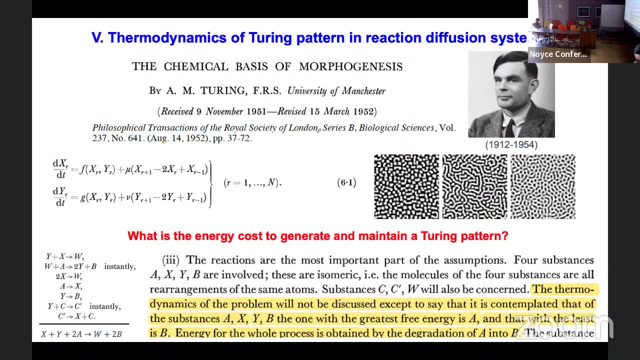 He actually considered specific chemical reaction. that embodies this right. So these are the x and y. You have w and a and b and c and c prime. c and c, prime are the enzyme. He didn't use the name enzyme, but that's basically. 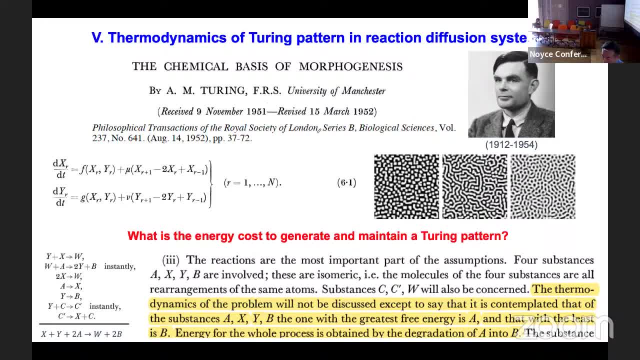 what it is. He said the reactions are the most important part of the assumptions. So if the x, y and b are involved, these are isomeric and the molecule of the blah blah blah blah substance b and c w will also be concerned. 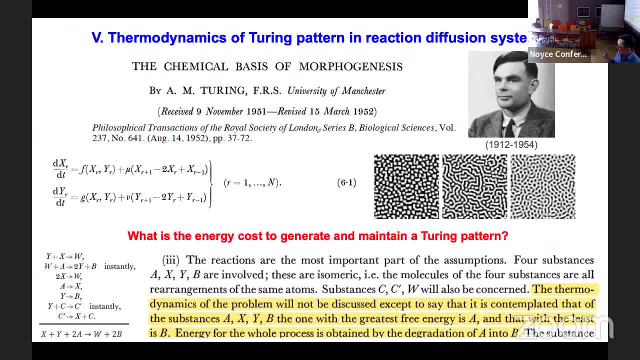 OK, then the highlighted part says the thermodynamics of the problem he's talking about. thermodynamics of the problem will not be discussed, except to say that it's contemplated. They like to use the word contemplated, Contemplated, that off the substance. 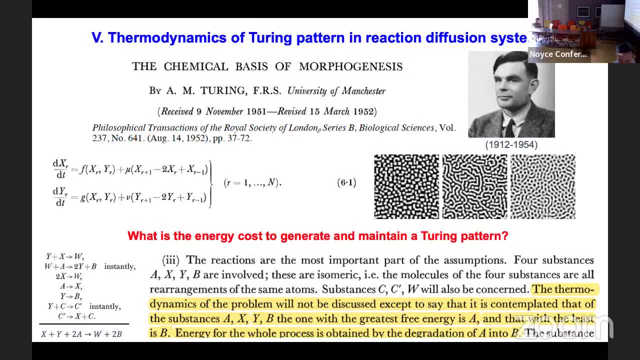 and the substance of the problem. So if the x and y and b the relevant ones, the one with the greatest free energy is a And that with the least is b, Energy from the whole process. he understands the process needs energy is obtained. 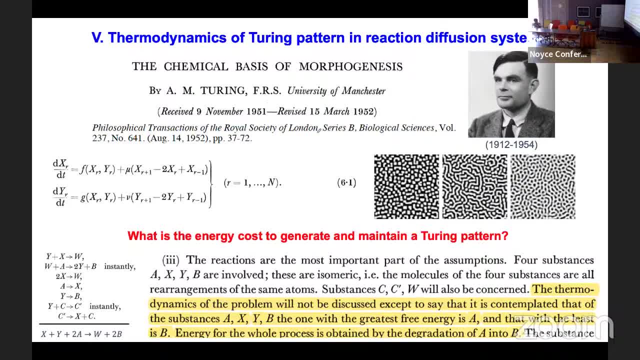 by the degradation of a into b. So if you sum up all the chemical reactions, what do you get? The x plus y goes to w, But 2a has to become 2b, So a becomes b. That releases the energy. 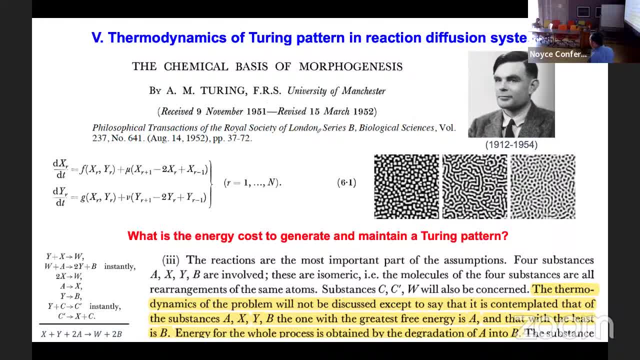 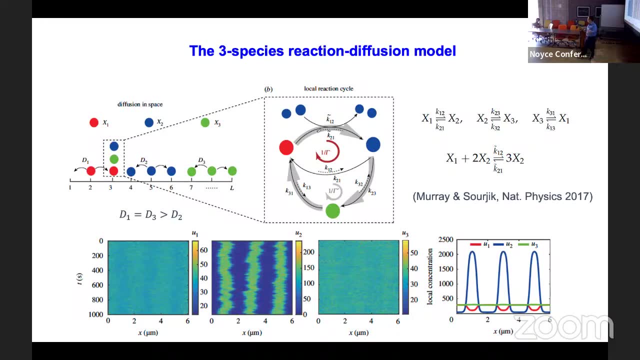 But in his mind that's the energy source And it drives the chemical reaction which eventually reaches the instability and then give rise to the pattern. I don't have time to talk about it, So we studied this question in more detail. We just basically put a footnote in this encryptive comment. 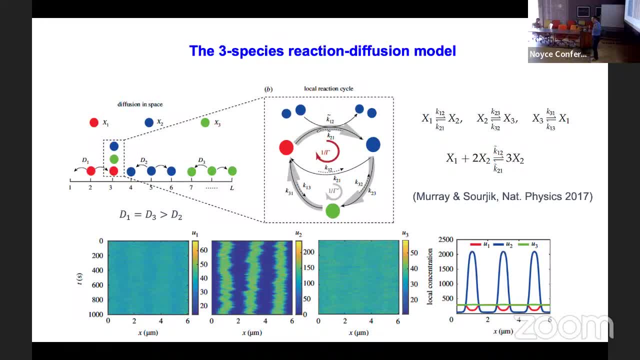 of Turing. Now we actually study for a particular system, like the three species reaction diffusion equation x1, x2, x3.. So basically the top line x1 goes to x2, x2.. These are isomeric. 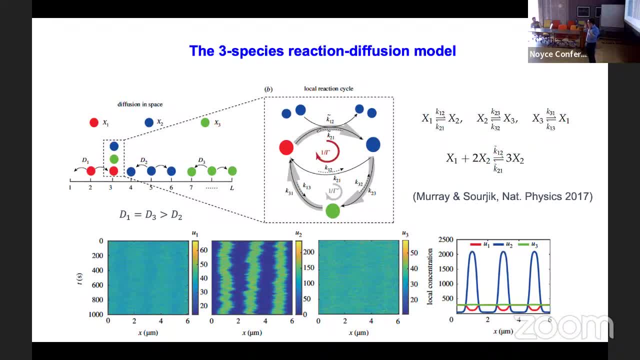 These are the same molecule but just different conformation. They go through each other through this cycle, So the chemical reaction is all described by this. This is actually very much like the Braselator model, which have temporal oscillation. people in the audience knows. 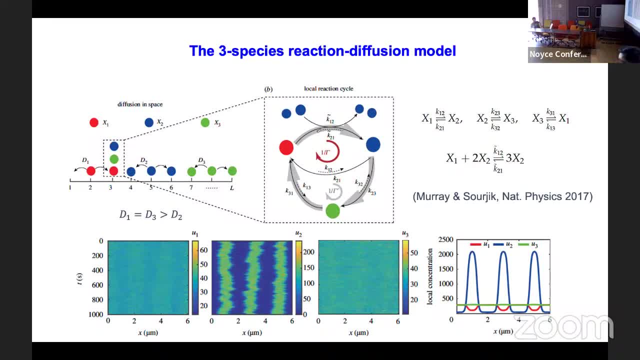 But then on top of it we put diffusion of all the species, And one critical ingredient in this is Turing's mechanism- is that the diffusion constant has to be different. The inhibitor has to be very quick, Diffusion is very high And the activator has to have a relatively slow diffusion. 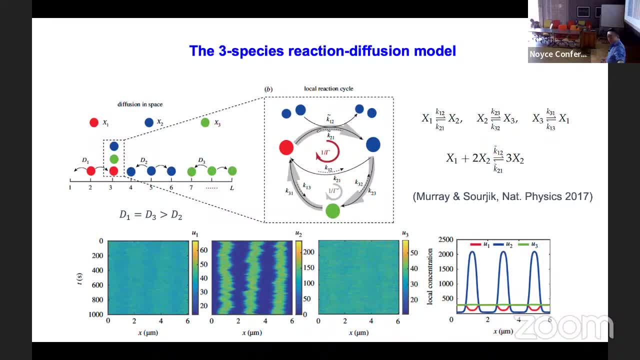 OK, so we put that in and the simulation shows that you form pattern. form this pattern. And now we actually also know, from thanks to Terry Ho, how to compute dissipation. correspond to this chemical reaction. We can compute the dissipation. 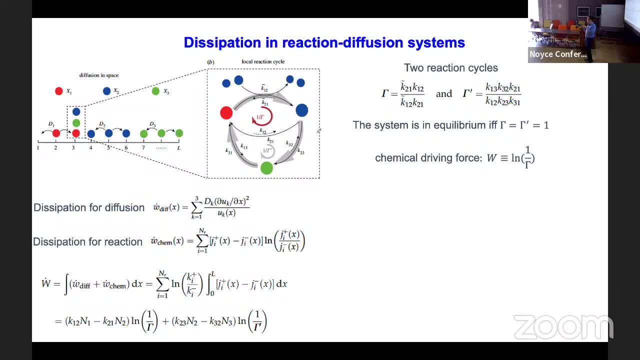 Right. So not only we can do that, we can decompose dissipation into the part of overcoming the diffusion and the part as it directly relates to the chemical reaction. OK, so we can do the same thing, that we can look at the critical line from no Turing pattern. 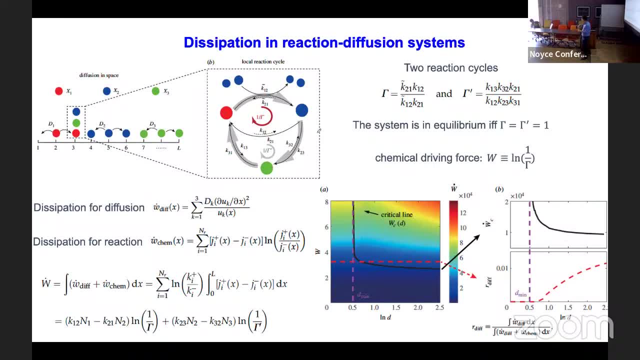 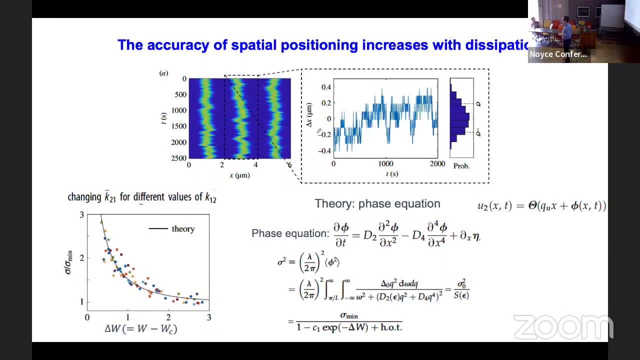 to Turing pattern and how much energy is cost and needed to go there. So one thing we discovered is that Turing pattern needs a minimum of energy, But usually, typically, the energy input is much higher than that. Why is that? The additional energy above onset? 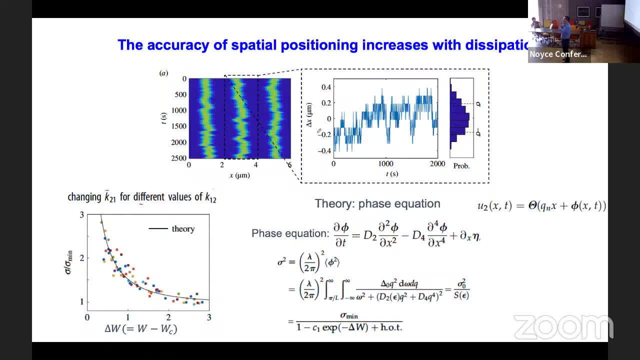 is caused to suppress the fluctuation of the spatial pattern, Because for a finite system, even though you can create a pattern, the pattern actually fluctuates a lot. Actually, in some cases this is very detrimental to the biological function. So you don't want that. 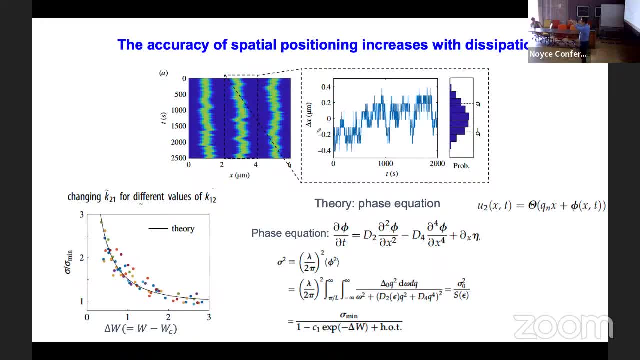 So we can characterize the fluctuation of the Turing pattern by the standard deviation of the pattern over time, sigma. And you look at the sigma dependence on the energy dissipation. So here is the critical energy cost for you to have any pattern at all. onset of the pattern. 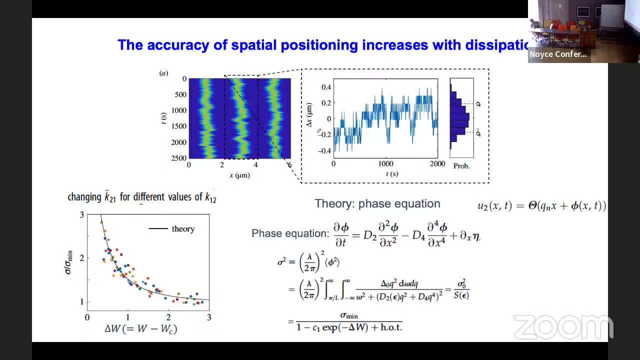 But you keep pushing it. what you find is that, instead of creating the pattern, this additional energy is being used to suppress the fluctuation in the finite system. So that's what we found. So energy is not only useful for generating the pattern itself. 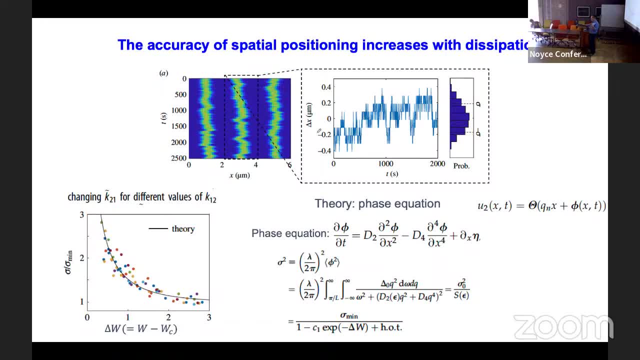 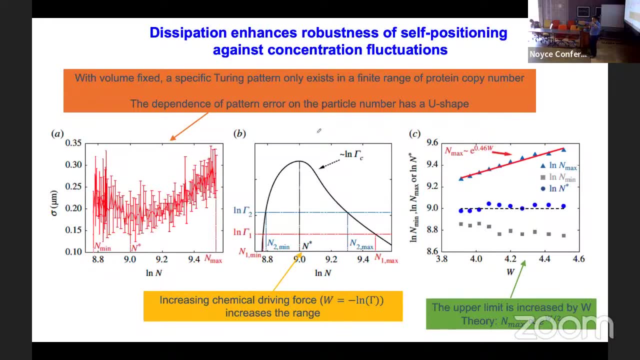 but also maintain the high accuracy of the spatial degree of order. OK, So I also have other property like: enhances the range of concentration, Because in the single cell the concentration of molecule fluctuates a lot cell to cell. But nonetheless you want the Turing pattern. 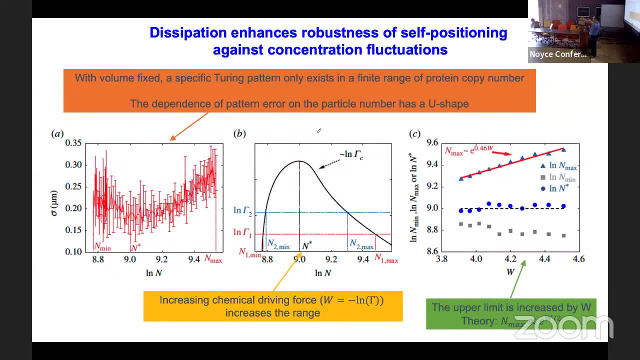 to exist in all these cells. So you want the range of Turing pattern to be large, And it turns out dissipation also allows you to have a broader range of allowable concentration in order for you to observe this pattern, So that's also good. 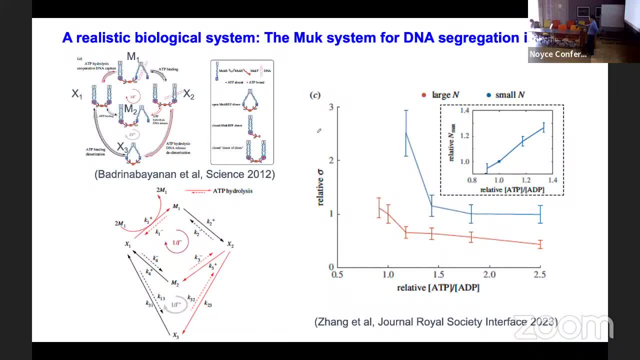 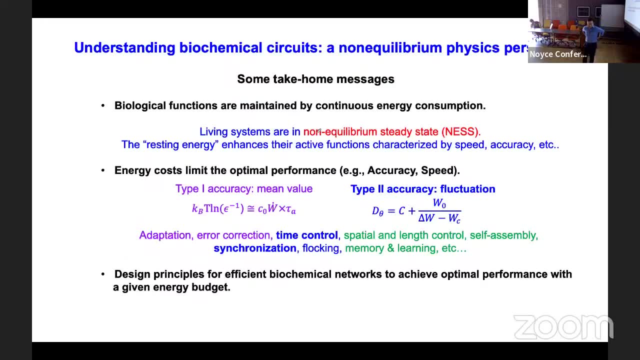 This seems to have implications. I think it's important for the MUC system, which is important for DNA segregation. I won't go into detail, Just some final remarks, some take-home messages. I think I would like to convince you is that. 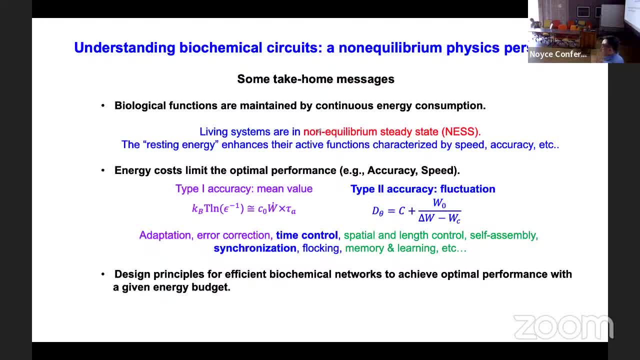 I think this is pretty trivial. biological functions are maintained by continuous energy assumption. So you think it's something that's just in the steady state, some harmless steady state, But underline it, It's actually this particular steady state, The living steady state is being kept in that way. 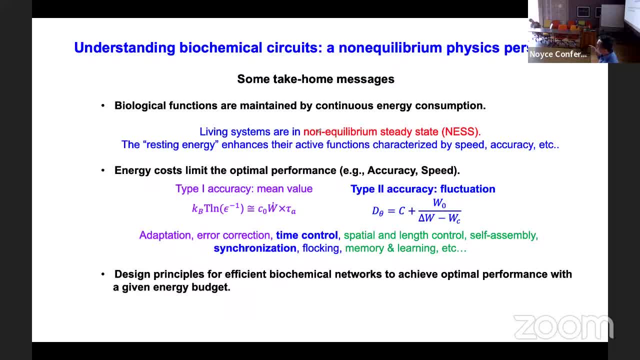 by continuous dissipation. And the amount dissipation is really related to the quality of the steady state, the quality in terms of its future potential to perform certain function or the function itself. But also the energy costs limit the optimum performance. So it sets a bound of how, if you 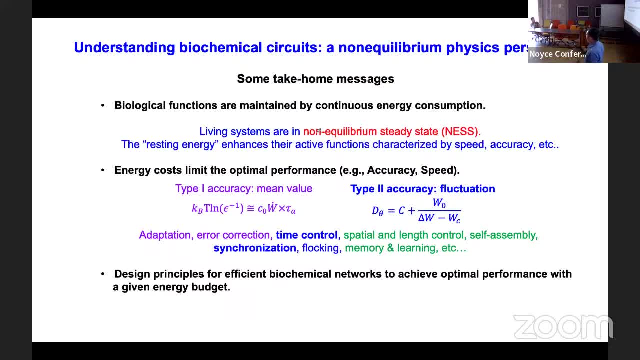 have this much budget, this much energy, this is the best you can do on the, or. I mean, if you have this much energy, then you can set a limit. So it sets a limit, So it sets a bound. Those bounds may not be realistic in the sense. 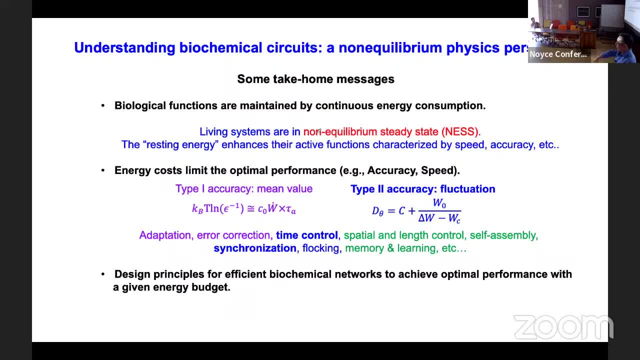 that they may be other constraints the biological system has to subject to, But this at least sets one bound from an energetic consideration. And finally, what I talk about, the bound, is really the case that it only sets a bound but didn't tell you how to achieve the bound. 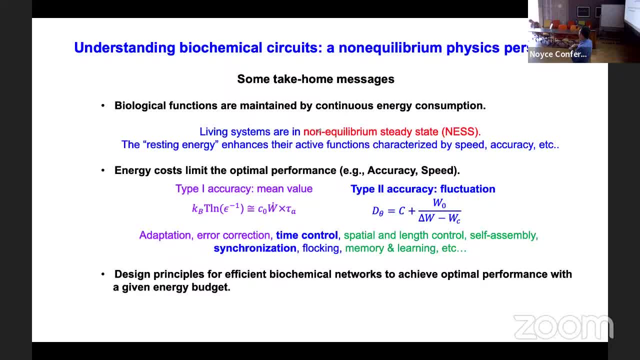 So I think a lot of study and work designed a circuit. if you want to play God, what kind of molecular circuit you want to build to actually achieve this function with the minimum cost? So this actually might be relevant for- maybe not directly for- real system, which is 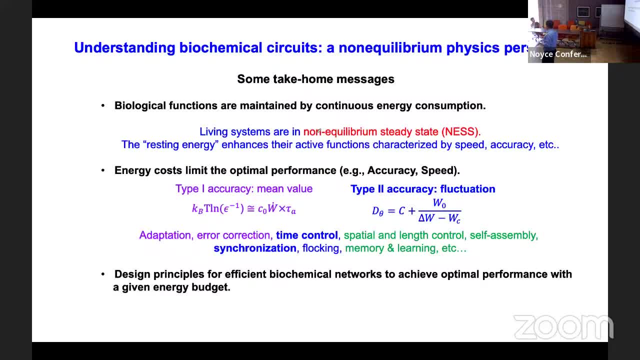 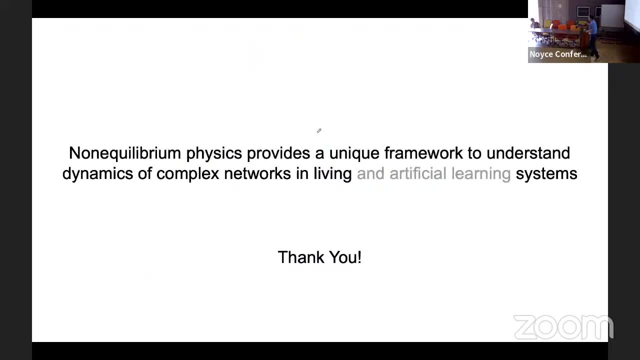 subject to other constraints, but probably relevant for synthetic biology. right, If you want to build a particular molecular machine that does certain function with a minimum cost in terms of energy, OK. so I end with a slogan that non-equilibrium physics, statistical physics, really provides a very unique framework. 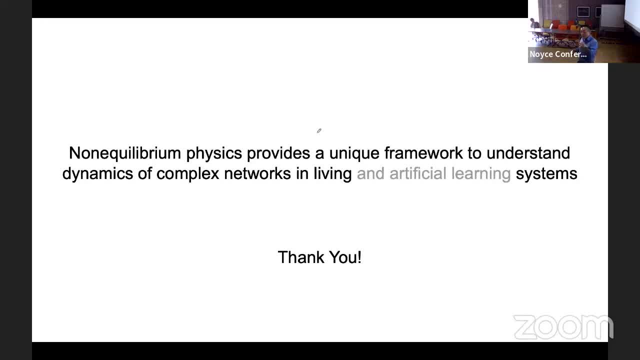 to understand dynamics of complex network in living system. In shaded I say artificial learning system. That's the subject of tomorrow, if you're interested. OK, thank you. Time maybe for one question? Yeah, Yeah, thanks for the really wonderful talk. 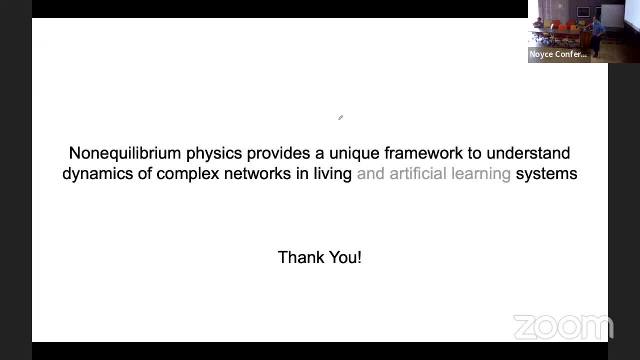 For this really beautiful clock that you showed. do you have ideas about what the evolutionary pathway to get there is? I mean because so often we're looking at machines like the ribosome or like this that is the endpoint of this wonderful evolutionary trajectory. 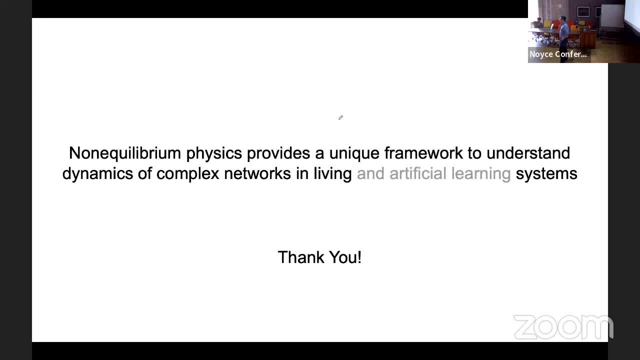 They're highly optimized, They obey lambda error's bound, all of that. But do you have ideas of what the immediate clocks might look like? Yeah, so back to my. I didn't make a comment before, So they are. so they are chi a, chi b, chi c, right? 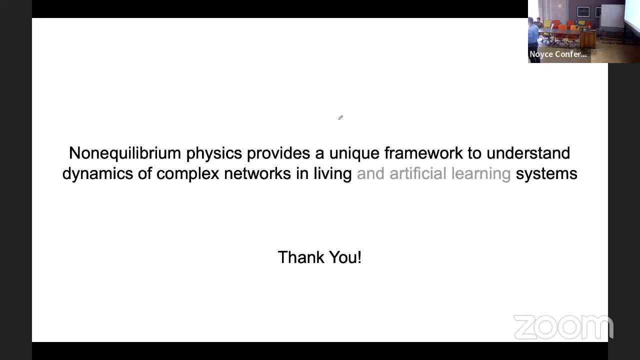 Three components, But so the I think earlier event, earlier clock. but it's a passive clock, what they call the hourglass clock. Basically, you have to turn it one side or the other to make it run. It only have b and c, no a.